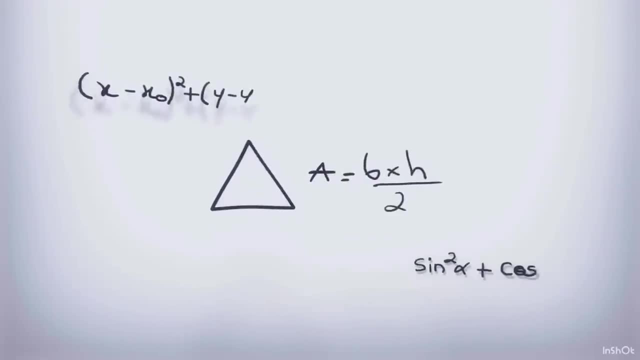 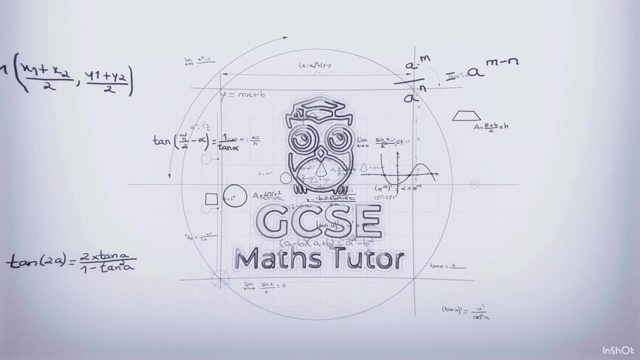 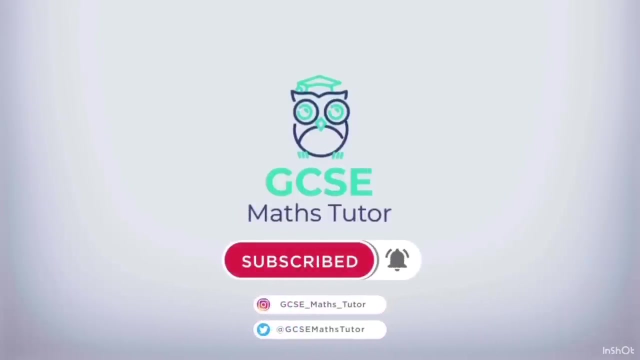 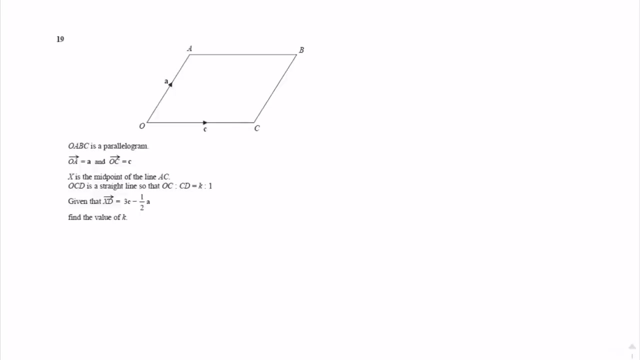 Okay, so in today's video, I'm going to be doing something a little bit different. We're going to be having a look at these real top-end vectors. Now, what I would suggest is that you obviously look at the previous video, which I'll link in the description, looking at vectors, because 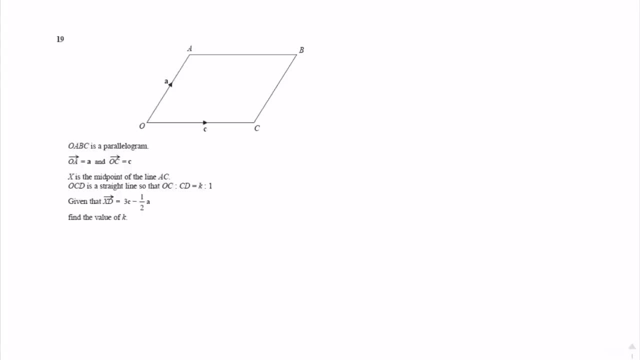 this is a real big step up in terms of the vector topic. Okay, so you probably have known some of these questions in the past, but they are some pretty tricky questions here. so this is really the top, top end of grade nine and obviously vectors is a difficult topic anyway, so we're 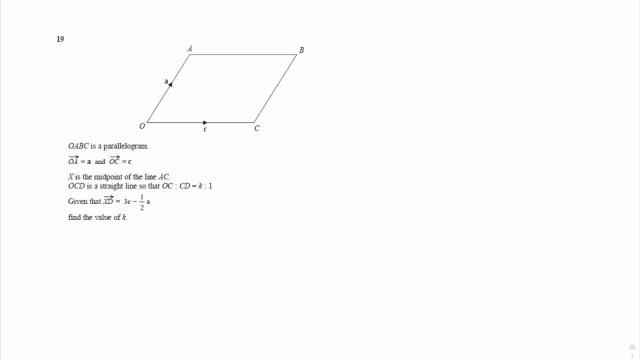 going to have a look at all of these different types of questions. So grab a piece of paper, grab a pen, try and draw these as best as you can and make some notes. What I would suggest is having a go at the questions, seeing how far you get and then watching my little explanations of. 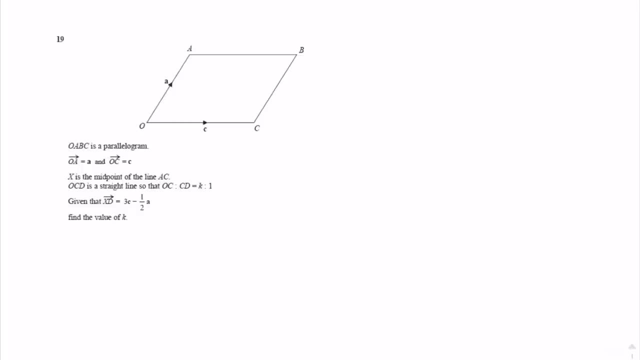 these. So I'm not particularly going to give you any questions to practice, like normal, but what I'm going to do is just go over five of these questions here that have been quite tricky and we'll see how we get on with them. So for this question here it says AOBC is a parallelogram. 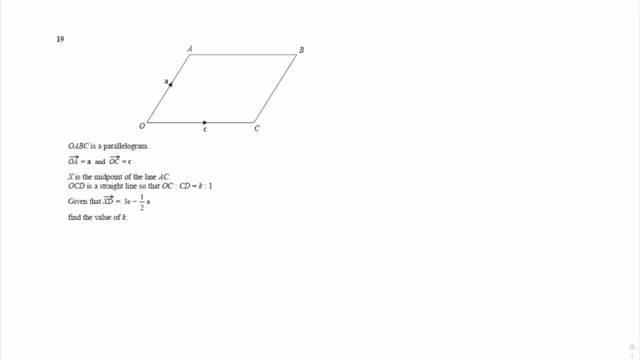 and it gives us some vectors: O to A is A, which is drawn on the diagram there, and O to C is C, which again is drawn on the diagram. It says X is the midpoint of the line AC. Now, straight away, we don't have a line AC, so let's draw that in. So A to C is here and X is the midpoint, So right. 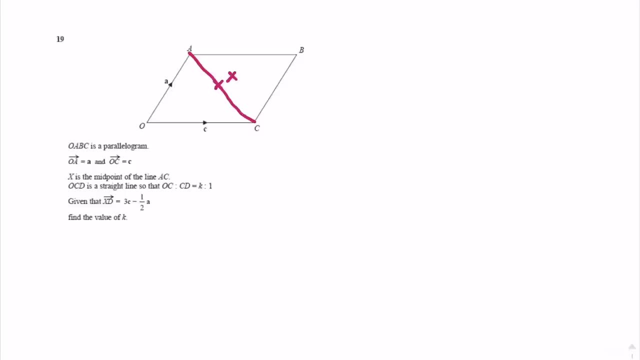 the middle there, that's X. Then it says OCD is a straight line, so that O to C, C to D is K to 1. So OCD- Now we don't have a D, but it's the continuation of the line OC. So somewhere over. 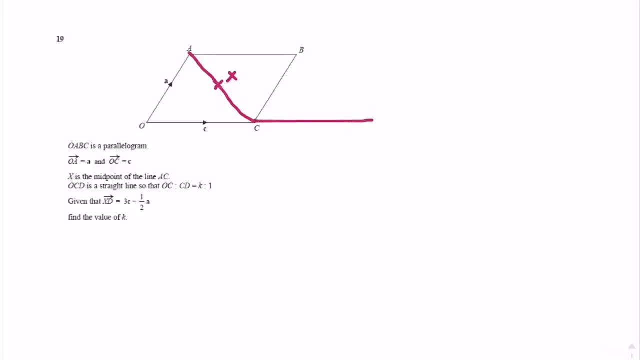 here. we don't know how far it is. we've got this point D. Now let's just say it's over there, Okay. and it says that's in the ratio K to 1. So O to C is K to 1. Okay, there we go. Then it says: 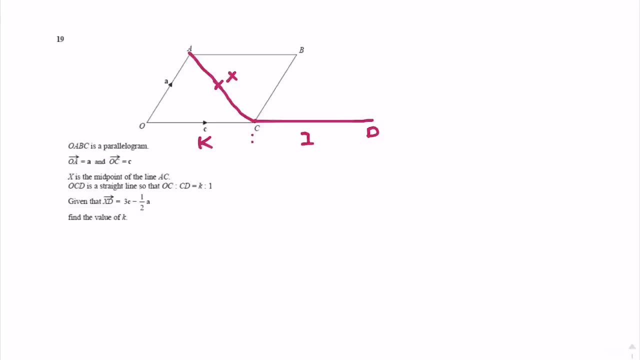 OCD is 3C minus a half A. Find the value of K. So from X to D, which we can join in, let's do that in a different colour, from X to D. There we go and in that direction is 3C minus one half A There. 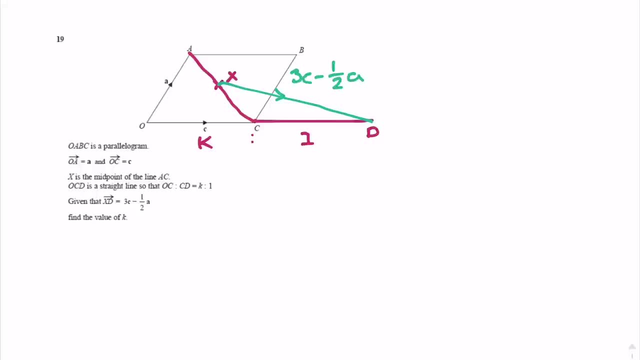 we go and that's the vector. That's all the information in the question that's given to us. So, first things first. what we need to do is we need to find this value of K Now we need to have a look at this diagram and think about what it is that we're actually going to do here. Now, what we 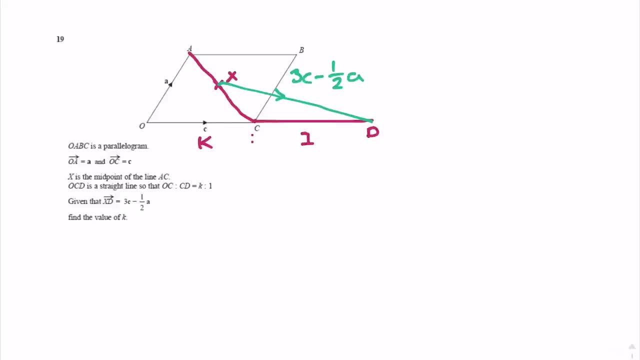 need to do is try and find our own root from X to D. Obviously, we've been given the fact that it's 3C minus a half A, but if we can find our own root, we can see if we can make it match that vector. 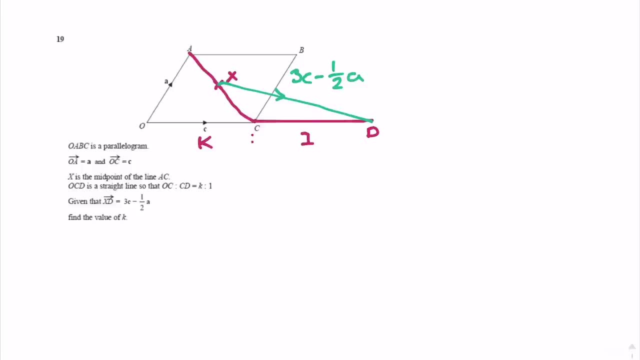 there 3C minus a half A. So think about how we could actually get from X to D in a different way, not just following that green line that I've drawn in. We could move. let's have a think we could move down C and then across here and try and get that vector there to match. 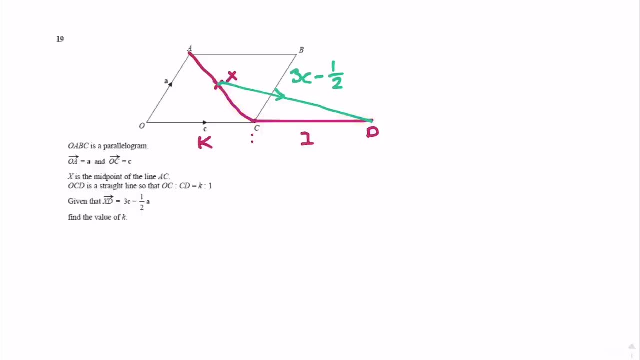 or potentially we could actually go. well, I think I might have just erased something there. Yes, I have a look. it was that A There we go. Or we could actually go upwards up to A down here. oh, there, we go down to here, and then again all the way across. So that's another route that we 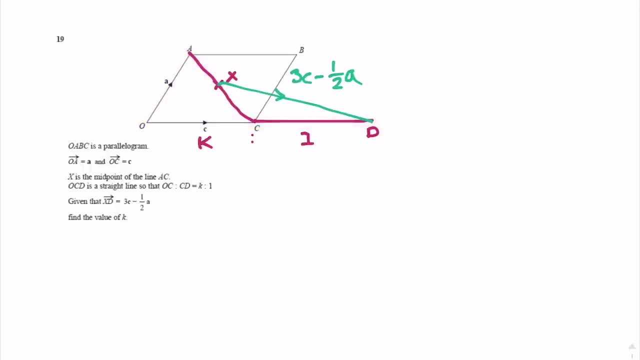 could take. So that's what we're going to have a look at. We're going to have a look at actually finding one of those routes. Now let's swap to a different colour. First of all, let's have a look at this line, this line A to C. Okay, so, in order to move anywhere in either of those routes, we need 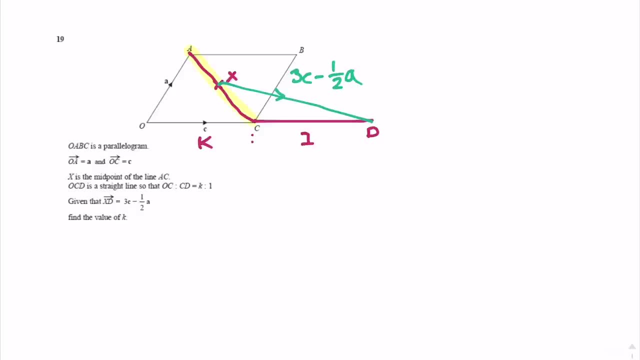 to be able to move halfway through this line. So in order to do that, we need to know the full line. let's label this So: A to C. what's that vector there? Now, to get from A to C, we can go down through there, backwards through A, so minus A plus the C, And you can write that as minus A plus C. 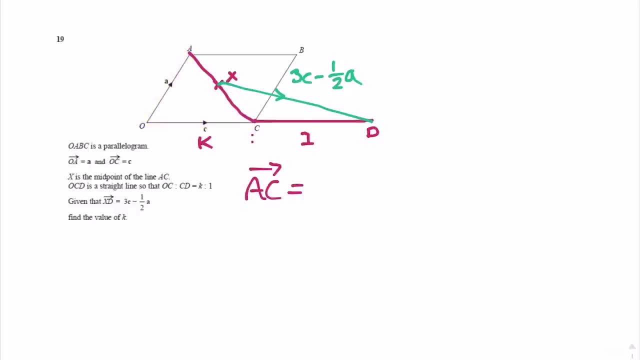 or you can swap them around. I'm going to keep it as just minus A plus C, So minus A plus C, and obviously you can write that as C minus A, if you want. Now let's have a look at moving through half of that, as X is the midpoint, So we can go from A to X rather than from A to C, So A to X. 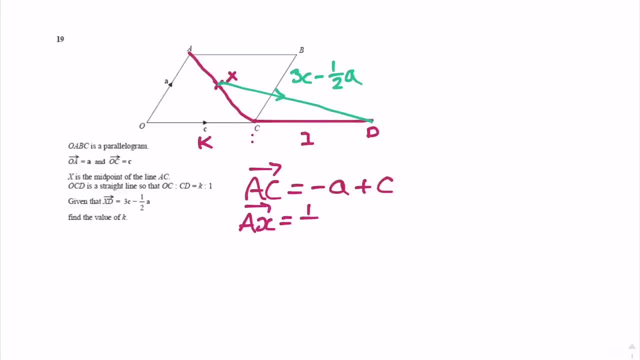 will be half of that. So if we want to do half of that, we just times it by a half, which I'll put as a half. lots of minus A, plus C, And we can even go ahead and expand that if we want. So we can say: 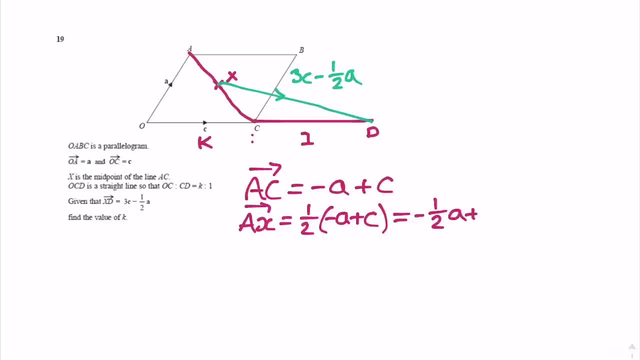 minus a half A plus one half C, There we go, just expanding that bracket by that half at the front there. Next step: let's have a look. how could we get from O to X? Okay, so we had a look at part of that journey. Let's have a look. how could we get? we now know how to get from A to X. Let's have a. 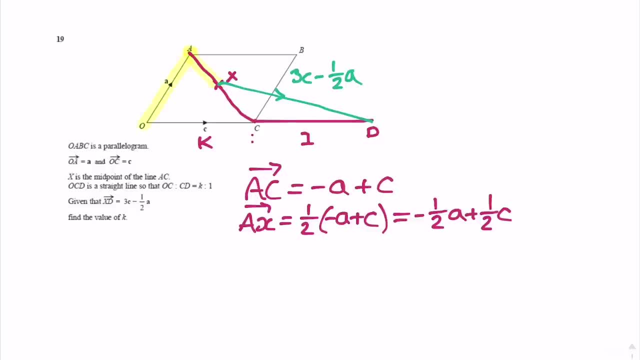 look now how we get from O to X. So moving up here And then down to X. Okay, so O to X, Let's write this one in. Okay, so to get from O to X we'd have to do another A. Okay, so we have to move from O up to A. That's. 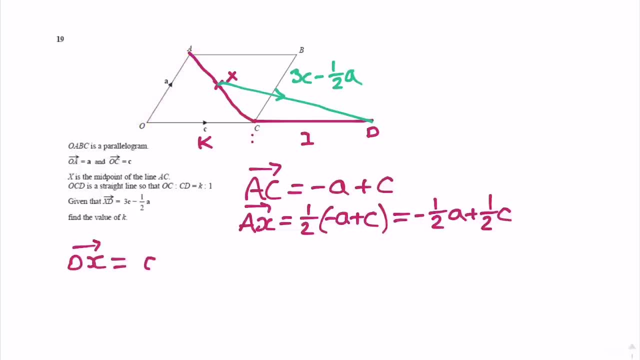 a vector of A. So if we do A and then add in our A to X vector there, which we've just done over there, So minus a half A, So A, minus a half A, plus a half C, And if we simplify that, we've got. 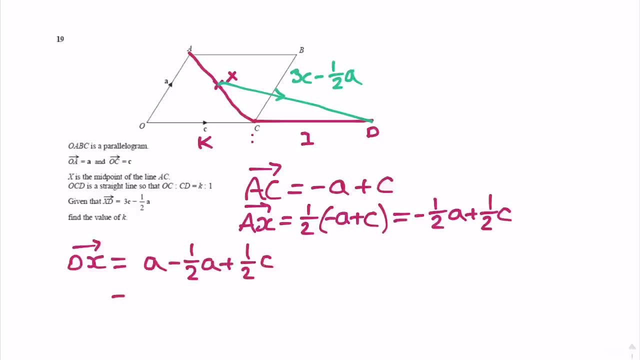 one A. take away a half A, which leaves with positive a half A. So that's going to be one half A plus one half C, And there we go, And that's our vector: O to X. Now let's have a look at how we get from O to D. To get from O to D, we would have to go from O. 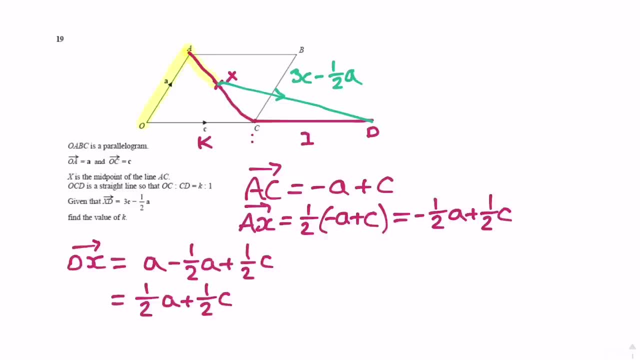 up to A, which we can do From A down to X, which we've got. We've got O to X, And then we could move from X to D down that way, And that would give us our vector from O to D. So let's have a. 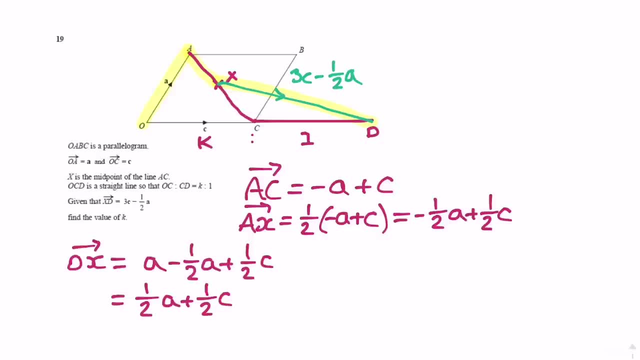 look at what that actually gets us. Let's get rid of that Now. we've already got O to X. So we're going to have minus half A here, That additional part of the vector that we're going to move. So let's get rid of all of that Now. from O to X. we've already got, We've got it down here And 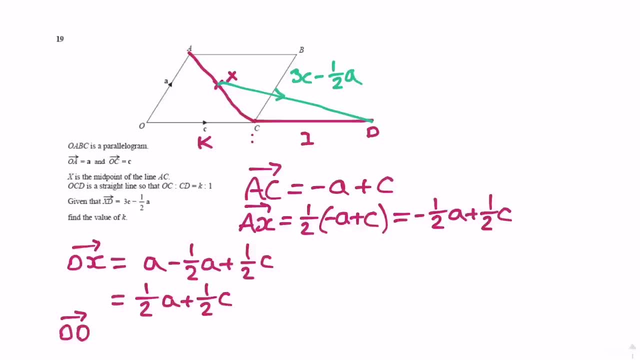 this time we're going to go from O to D, So we're going to add in the additional vector there in green 3C minus half A. So we've got the half A just above here, Half A plus half C, And we're 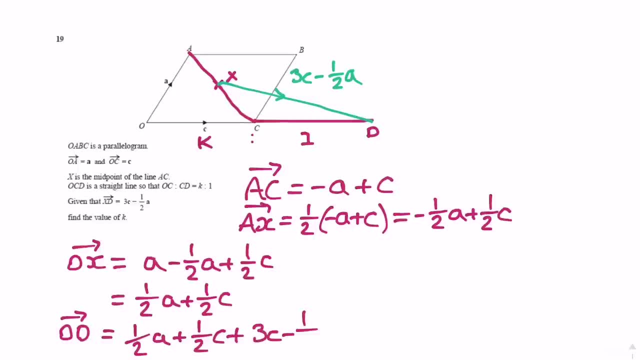 going to add into that the 3C minus one half A, And we've got to simplify all of this. and let's see what we get Now. we've got a half A at the start there And we're going to minus half A. So 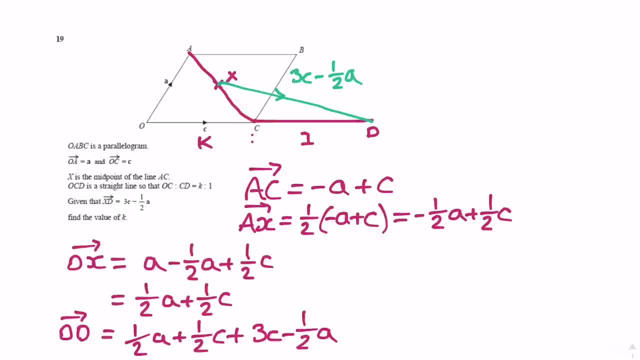 A's are going to disappear. So that's got rid of the A's, And then we've got a half C here, Add a 3C And if we add those together that gives us a combined vector there of three and a half C. 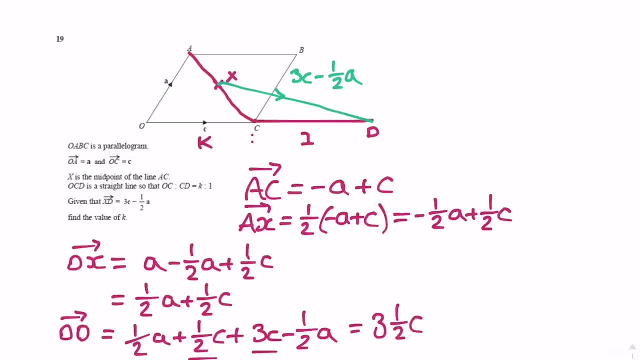 Again, which you can leave as top heavy or in decimal form if you want. But we've got 3.5C there as our vector- O to D, So to get from O to D it's 3.5C, So we can just leave it as a fraction. 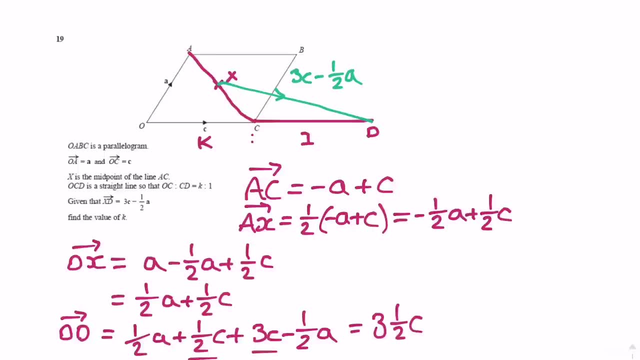 Now, if you have a look at the vector O to D, at the moment we know to get from O to C is a vector of C, Just 1C, And then from C to D is another amount of C's, as it's going along in that same direction. 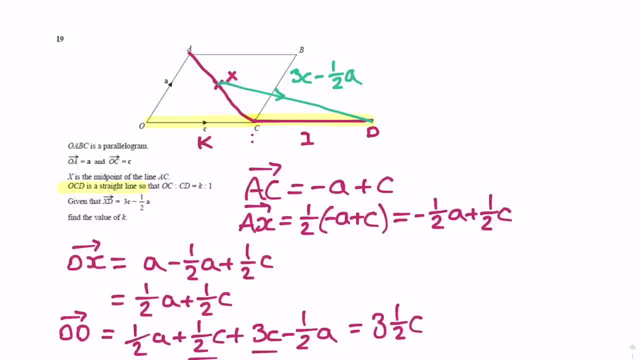 It's a straight line, as it tells us in the question here. OCD is a straight line. It has to be an amount of C. Now what we've figured out down here is that that full amount is 3.5C. Now at the. 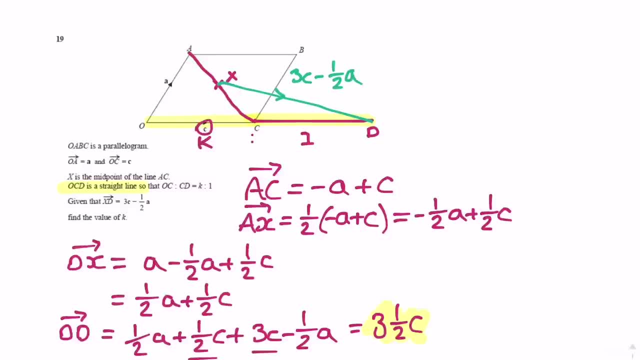 moment. obviously we know that there's one C here, So the C to D vector, So from C to D, has to be another 2.5C to actually make sure it makes that full 3.5C that we've just found. So that 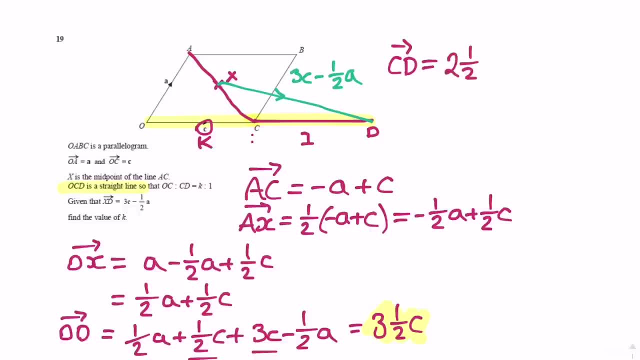 must be C to D, must be 2.5C or 2.5 lots of C. So at the moment we've got that and if I get rid of this little vector, this little ratio- sorry, down the bottom At the moment I've just got rid of. 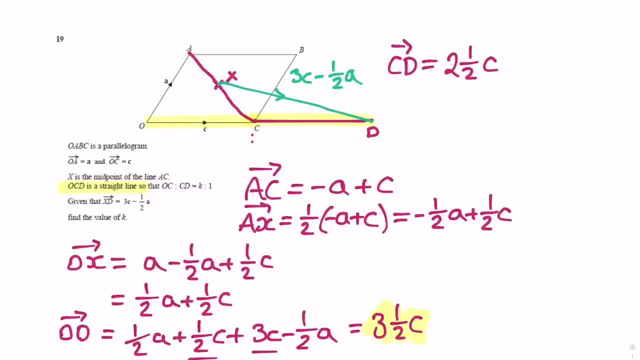 that I don't even know what was drawn there. Let's have a look. Oh, it was a highlighter, Okay, so let's get rid of that. So, at the moment, what we have is: let's get rid of this. There we go, What we have. 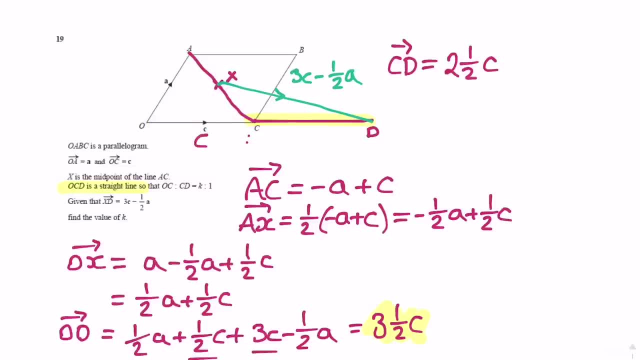 is 1C here to 2.5C's here. There we go, and that is our little ratio there: C to 2.5C. So if we write that as a ratio from O to C- which is what we're looking for- to C to D, There we go. At the moment it's 1C, which I'll write in. 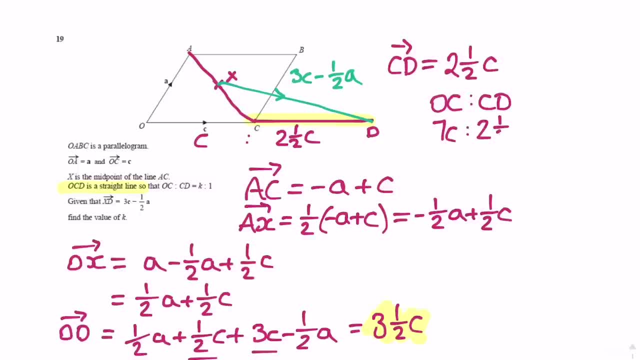 the 1. 1C to 2.5C. There we go, 1C to 2.5C, and it says it wants that vector- sorry, that ratio- in the ratio K to 1.. Okay, so we want to figure out how we're going to make this right hand side. 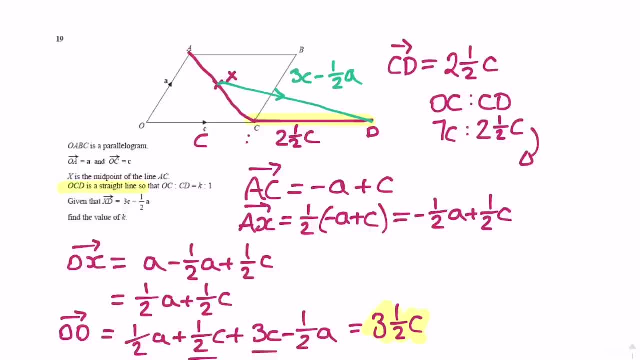 be a 1.. So let's think about how we're going to make this right hand side be a 1.. So let's think about how we actually go about doing that. Now, in order to get that one on the right there to become 1, we have to divide it by 2.5.. Okay, so we have to divide 2.5C by 2.5.. So let's write here: 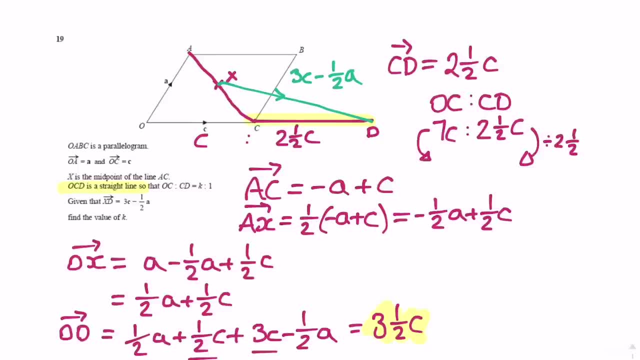 divide by 2.5, or divide by 2.5 and again, we're going to do that to the other side as well. So divide by 2.5 and that gives us 1 on the right hand side, like we were looking for Our number. 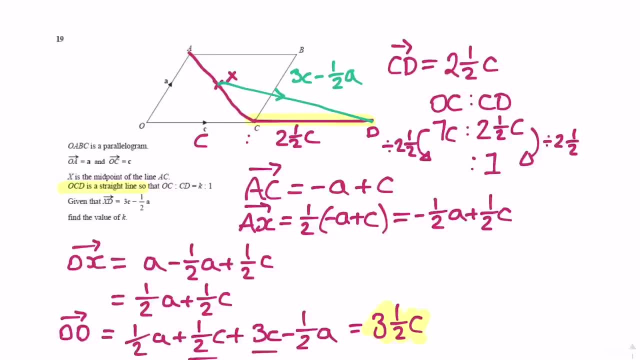 1 there, and we just have to do 1 divided by 2.5.. Now I'm going to do that just down here. Think about how we'd do that if it was non-calculator, which this question is. So let's have a. 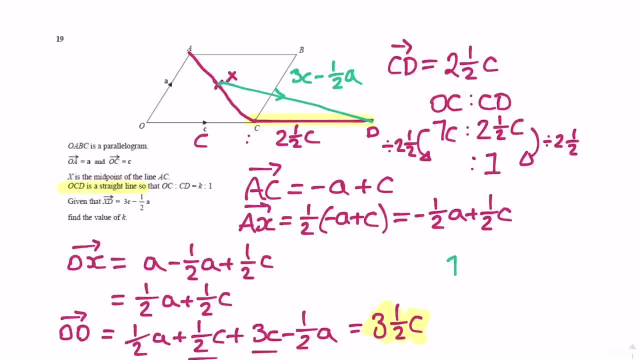 think We've got 1 and we're going to divide that by 2.5 and we're just going to follow our normal rules of fractions for this one there. So obviously when we're dividing or timesing or adding with fractions, we need that to be top heavy. So actually I'm going to do 1 and I'm 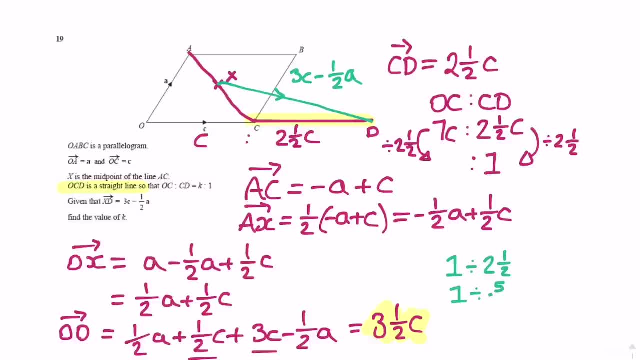 going to divide it by make that top heavy, we've got 5 over 2.. So, again following our rules of fractions, we've got 1 and we're going to times it by 2 fifths. Now, 1 times 2 fifths is 2 fifths. 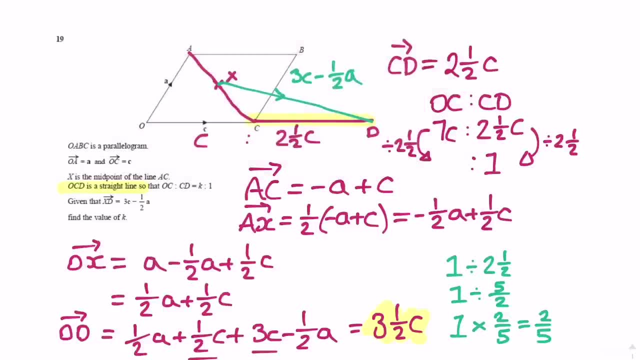 So bringing that back up into our ratio there, 1 divided by 2.5- we've just figured out- is 2 fifths. So our ratio there is 2 fifths to 1.. That's going to be quite important, So obviously. 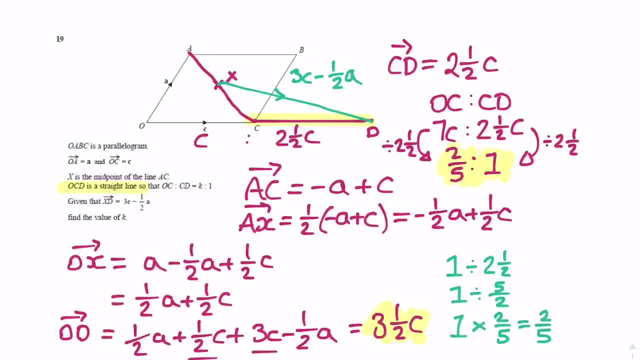 it says it's in the ratio k to 1.. That is now in the ratio k to 1.. Our k is 2 fifths, So our value of k is 2 fifths. We just need to write that somewhere. Let's write it right here in the. 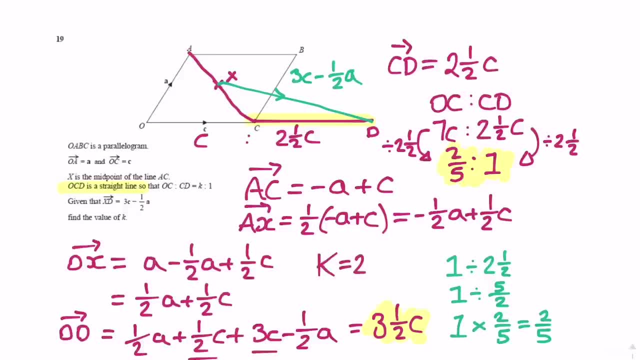 middle. So k equals 2 fifths. There we go and that's the final answer for that question- Again, quite a tricky one. It's about figuring out actually what you're actually trying to do when you're just trying to do these questions. But there you go. there's the answer and the idea. 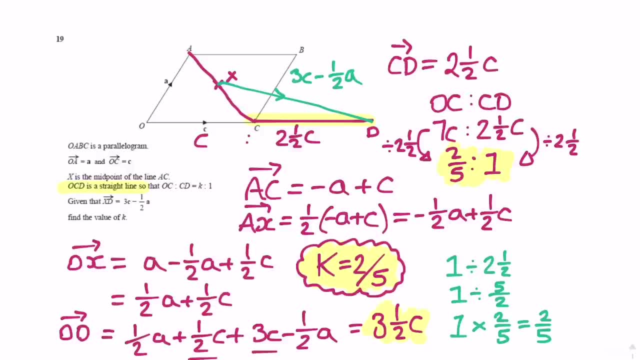 about how you go about this: Finding that vector from a to d using some of the vectors that you can find and can use, and obviously the one that was given to you there, and then comparing it to that full line o to d there, obviously in a different way. So we looked at two different. 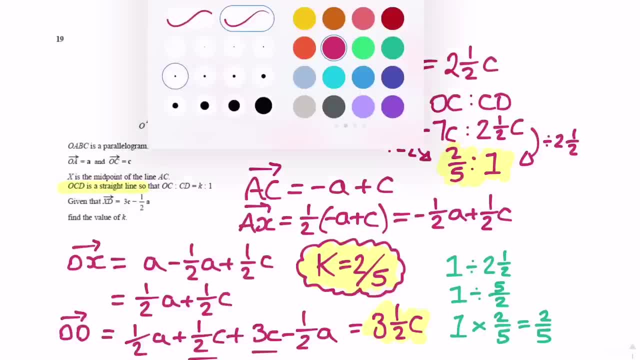 ways. Let's just get rid of that and bring this back in. So, in terms of what we did, I can just draw this final line back in there. There we go. We looked at two different ways. One was the full line there, o to d, which we looked at at the end. 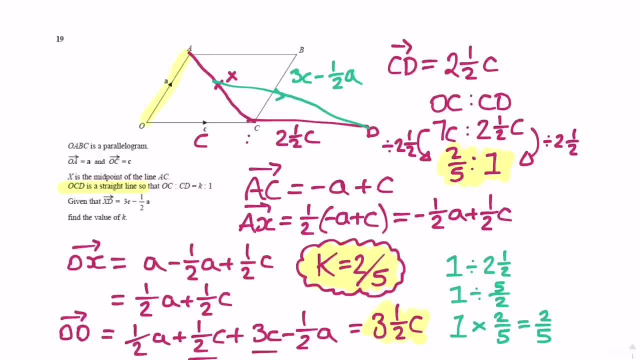 and also we looked at the root o to a, a to x and then x down to d, using the vectors that we could actually find there that were given to us. So there was two different roots to get from o to d and all we've done is compared them and made sure that they match there using that ratio. 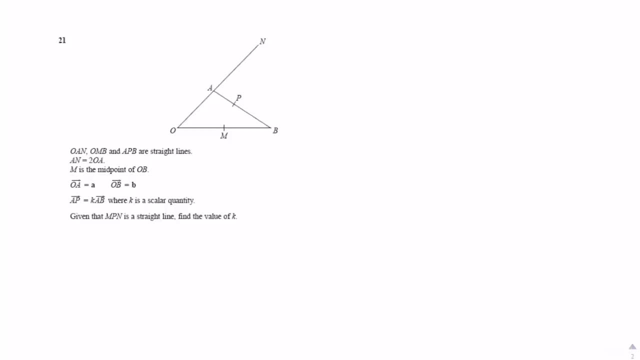 So that's that first question. Let's have a look at our next one. Okay, so this next question is a particular choice. It's a tricky one. Again, this was a calculator paper, but I'm gonna probably do this sort of in a non-calculator way- not that we really need a calculator as we go through this, hopefully. 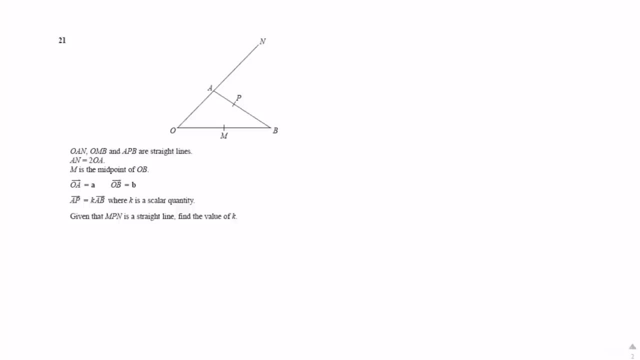 but let's have a look. It was actually on a calculator paper, but let's have a look. It says here that a to n is two lots of o to a in that second line there. So a to n- this one here is two lots of o to a. this one here. Now it says o to a is a. so if the other one's two lots of that, 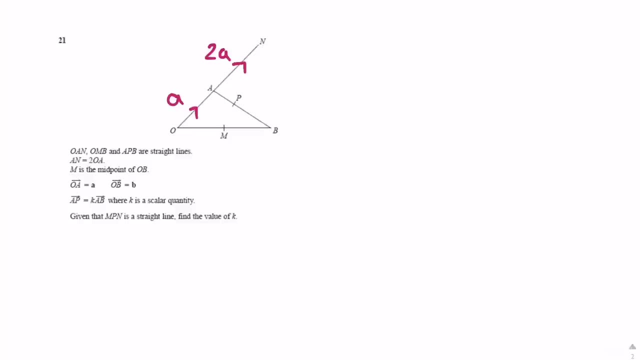 this must be two a. So there's the first bits of information we can get on the diagram. Then it says a to b is b and it gives us that point m there, which it then does it say anywhere. that's the midpoint. Yep, in the third line it says it's the midpoint. So if o to b is b, then each half here. 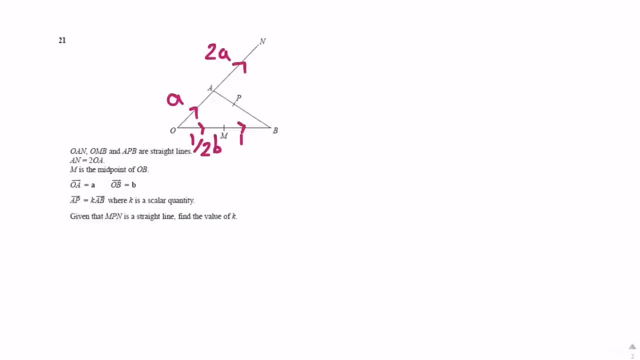 is going to be a half b, Obviously remembering there that the full length of the line is just one b. But there we go write that in considering that's a midpoint. Now it says a to p. is k lots of a to b? Why k is a scalar quantity, Given that m p n is a straight line following the value of k. 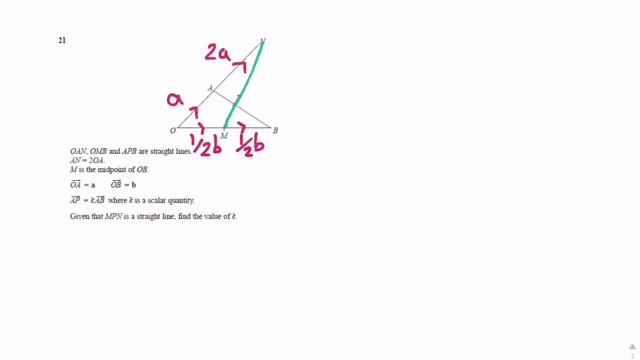 So it's just said m p, n is a straight line, so let's join that up. So b to n is a straight line and we're going to find the quantity there. So it says a to p is a certain amount of a to b. Okay, that's obviously a to p. there is only part of the line. 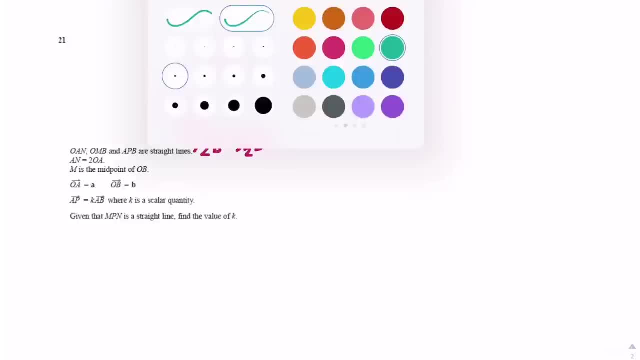 a to b. so that is going to be a fraction. So it's going to be a fractional amount at some point when we come to find that. Let's have a look at how we go about this Now. first of all, let's actually try. 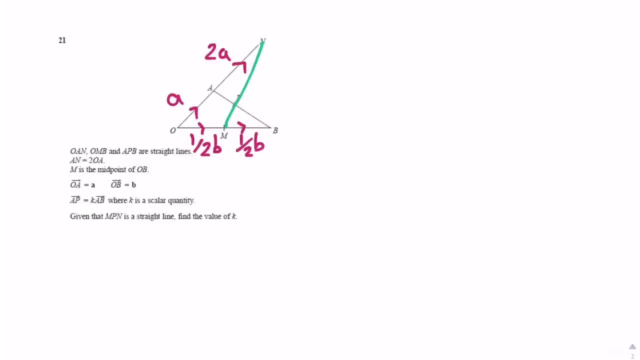 and find that full length of the line a to b, because it says that a to p is k, lots of a to b. So let's actually find the length of this line in terms of the vectors. Now we can get there from a plus these two half b's. so that's just going to be minus a plus b And let's write that down. 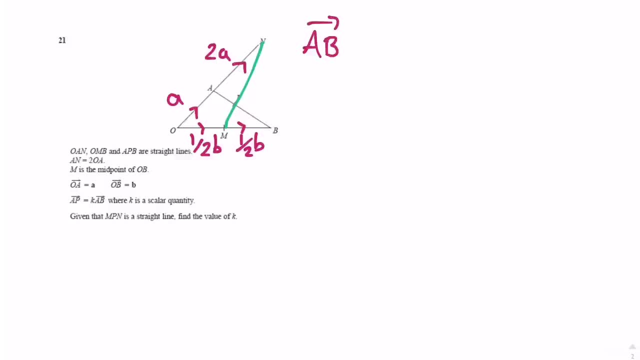 So from a to b, that is a minus a plus b. I'm going to swap it around this time: b minus a. Okay, now let's have a look at what we can find next. So what about that vector n to n, Can we? 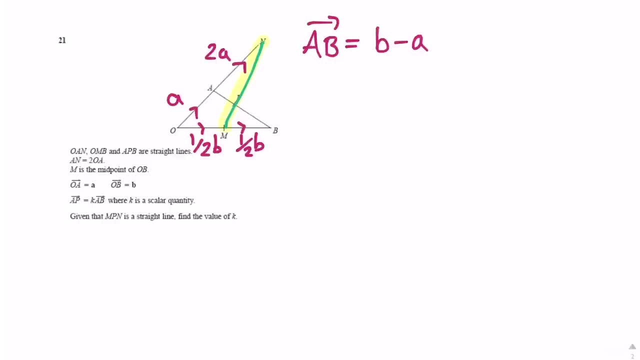 find that one. so, along that green line that I've drawn in, can we go from m to n and have a look at that one as well? So I can do that. I can get from m to n, and that's a lot of the time that these 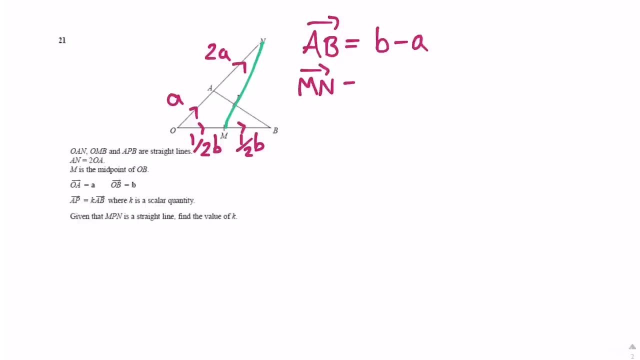 vector questions are about. Just having a look at what vector questions are about. So I'm going to vectors. can you find that aren't given to you? and m to n is not given to us? let's have a look and see if that helps us further down the line. so to get from m to n we can go backwards through the. 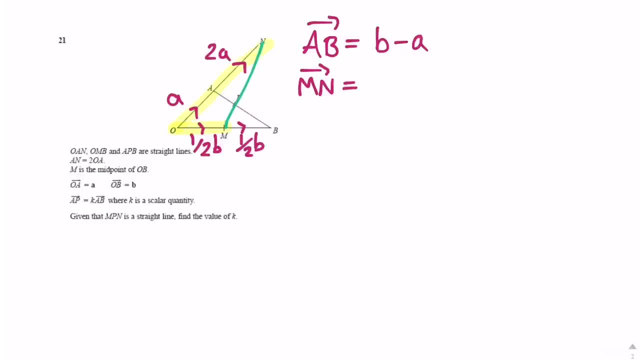 half b. so minus a half b and then positive 3a there. and let's write that in terms of: i'm going to swap them all around this time, so i'm going to do 3a first, so 3a minus the half b. there we go. 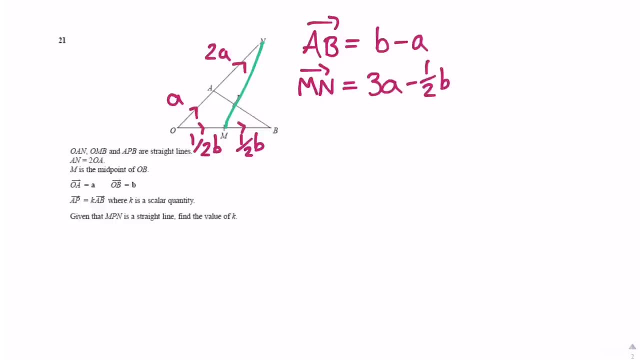 and that gets us from m to n. now let's have a think. can we find, can we get from m to p? then now, m to p, how would we actually get from m to p? because that's going to start helping us find how you know the length along the line that that is. so let's have a look. m to p at the moment, how would 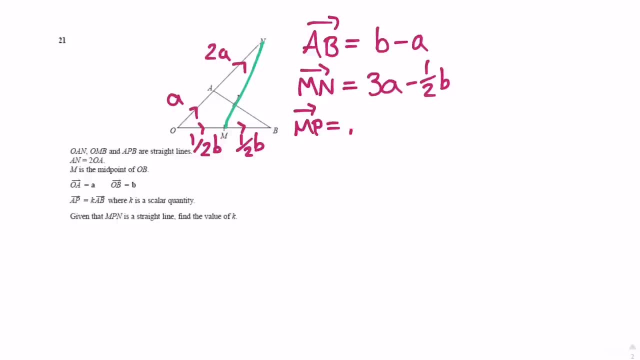 we get there, let's think about how we'd write this down so i can go from m to o. but let's write these down m to o, okay, that gets me obviously from m to o. then i can go from o to a, and then we can. 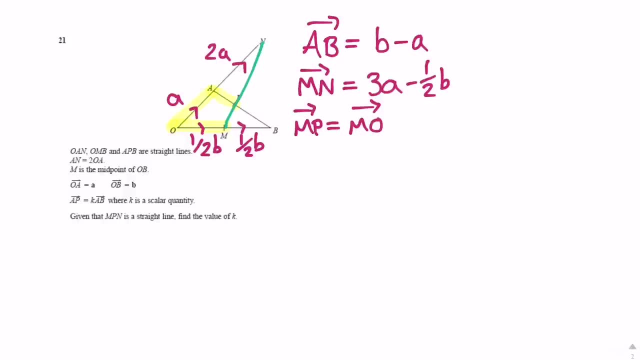 go down uh to the. uh, i've forgotten my letters behind it. now it's p, isn't it down to the p? okay, or we could go backwards, but let's just think about going that way, because we've got the vectors on that little root there, so i'll go from m to o, then i go from o to a, and then i would have to go from a to p, and let's. 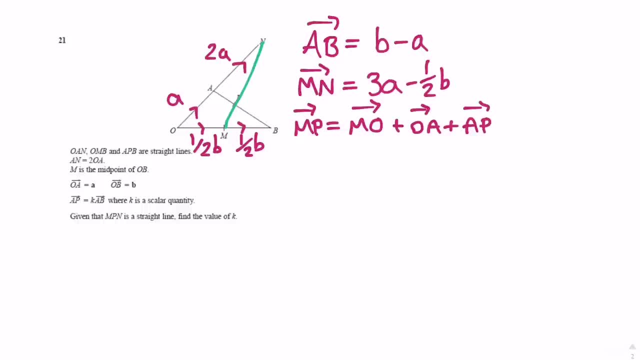 write that in there: a to p. there we go, and bearing in mind obviously that a to p is given to us in the question, it says that that is k lots of a to b. and we have a to b, don't we k lots of a to b. 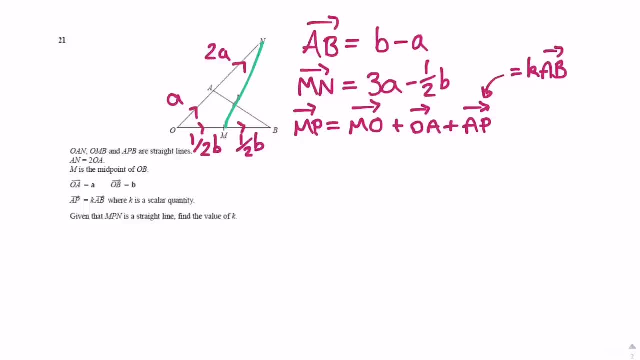 there we go, so we can obviously exchange a p for k, lots of a to b. so let's have a look at how we go about doing that then and writing that all in now, m to o is minus a half b, so minus one half b, and we're going to add to that o to a, which is one. 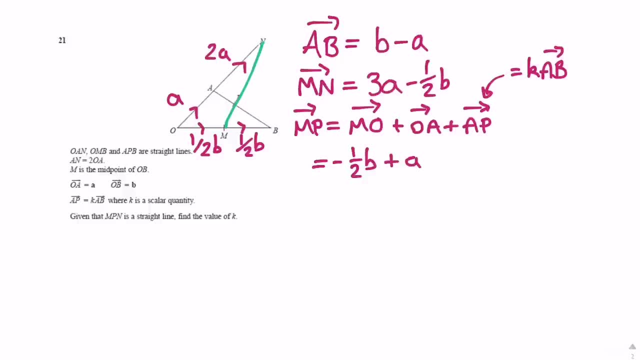 a, so add an a. and then we're going to add to that k lots of uh, that vector a to b, now a to b. we figured out in the first step which was b minus a, so add k, lots of b minus a. there we go and that's. 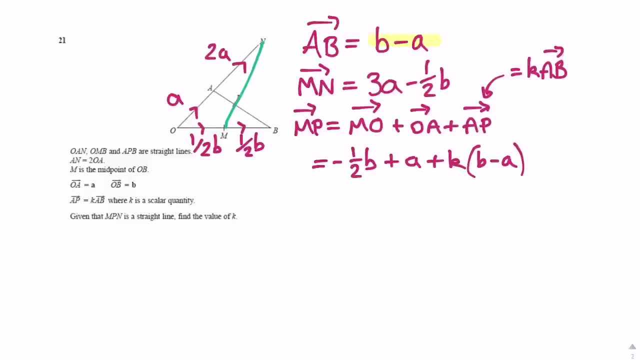 our vector m to p. now if we expand that out and simplify it all and see what we've got, let's first expand that bracket. so let's just rewrite this: we have minus a half b, and then we've got b plus a plus and then we have kb minus ka. now let's see what we get here. so if we simplify all, 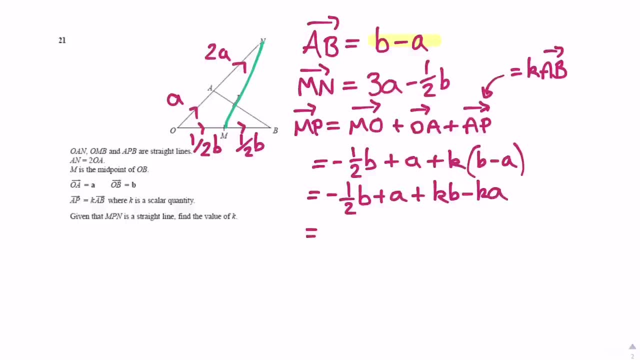 this down. let's see what we get. we have, and i'll tell you what i'm going to do when i simplify this, because obviously there's no pieces there that can join together, because at the moment this b piece has a k in it and this a piece has a k in it, so i'm just going to put the a pieces next to. 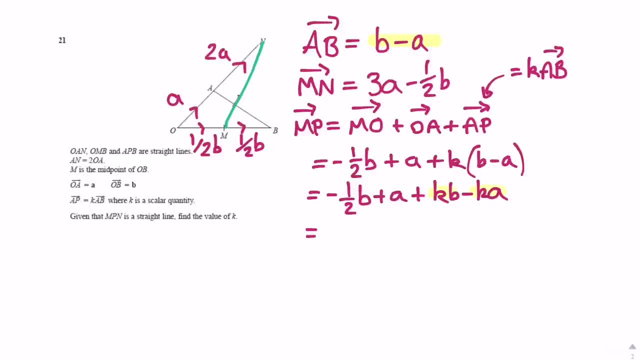 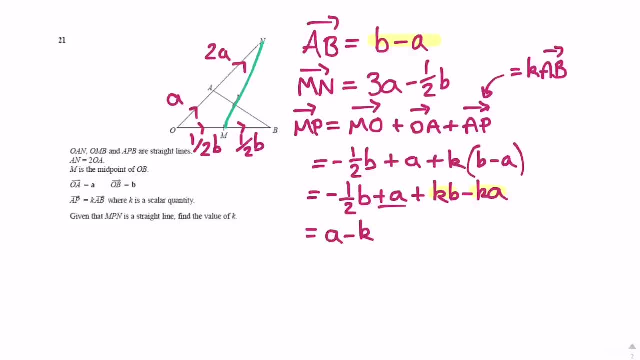 a and minus the ka at the end. so minus ka, that's the a's dealt with. then we've got minus a half b, which i'm getting just from the first piece there. so minus a half b and that's going to be plus kb, that little, the one that i've highlighted. obviously we could do the b's first. we could. 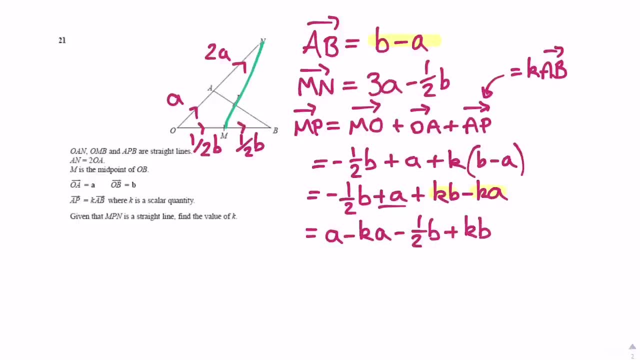 write them in different orders, but this is just the order that i've just seen the letters in, so i'm just going to write them in that order, okay, so that's the first one. now, at this point, um, when we've got these unknowns, okay, so we've got this unknown k here and this unknown k here and this. 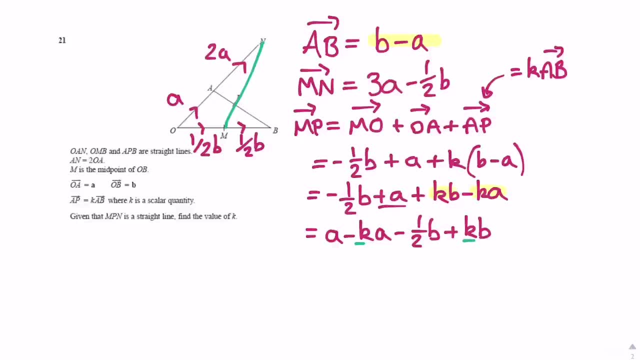 unknown k here. what we're going to have to look at now- because we've got this scenario- is we're going to have to look at comparing some of the coefficients here. so what i'm going to do is i'm actually going to um factorize this and i'll explain why. if you look at that length that. 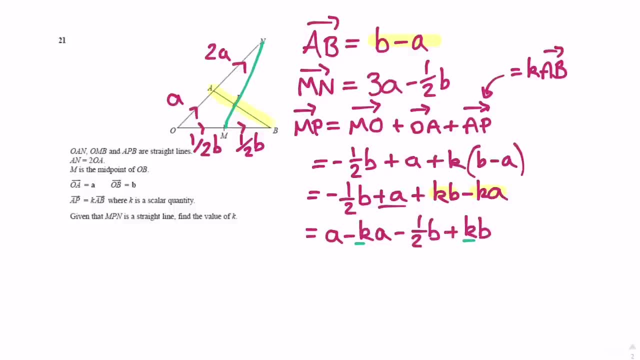 length: a to b. okay, this one here, a to b, there, if we're going to look at the vector a to p part of it, then the coefficients have to be uh, the same, okay, and at the moment we're looking at m to p. so we're going to have to look at the coefficients and those coefficients are going to have to match. 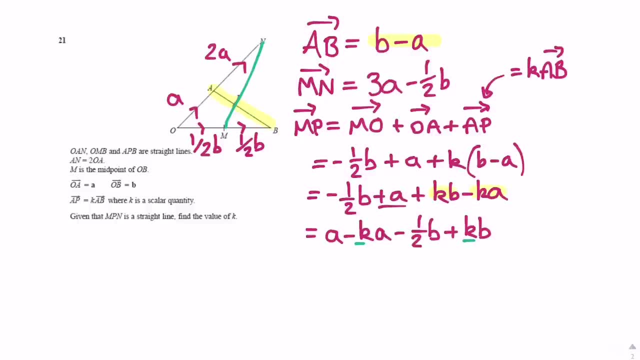 in in some sort of way, and that's what we're going to have a look at: actually comparing here and thinking if we can actually do that now in terms of the line itself. if we look at this line that we're moving along, we've got m to p. 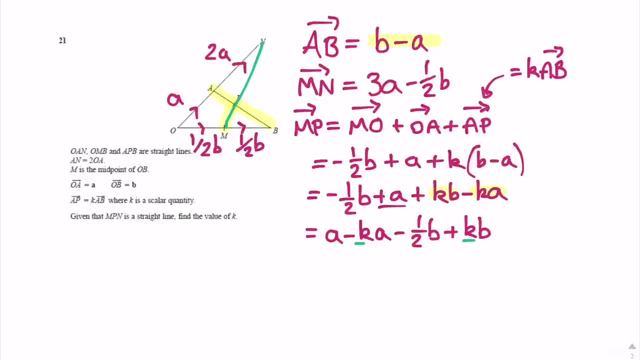 okay, which is here to here, and we've got the full length m to n. now we've already worked out the vector m to n. if i highlight that that's up here at the start. we've got 3a minus a half b and if you have a look at the coefficients of a and b there, the coefficient of a is three and 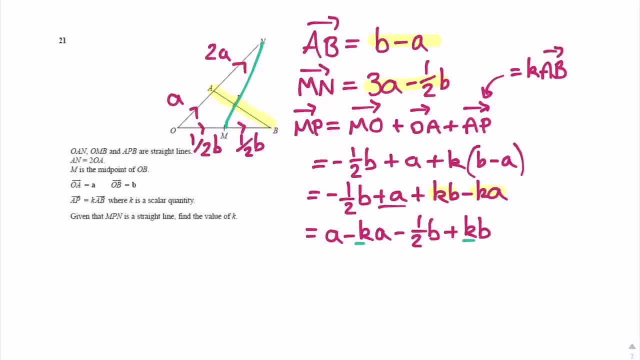 the coefficient of b is a half. now that means that just looking at the actual number in front of it, so forgetting about the minus, at the moment that coefficient of a has to be six times greater than the coefficient of b if you times a half by six. 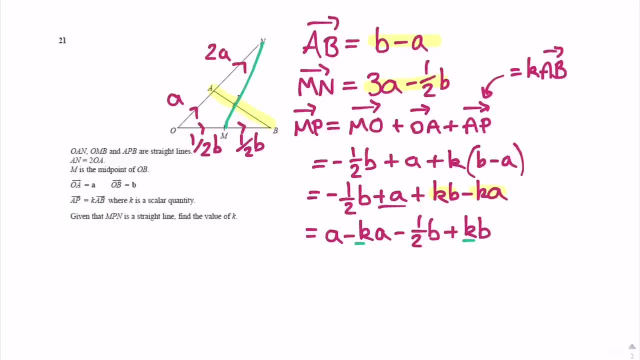 you get three, so that coefficient of a has to be six times greater. now i'm going to apply that little bit of logic at the moment when i have a look at actually what the coefficients of a and b are at the moment down the bottom here. now, if we factorize this, we can actually have a look. so if i 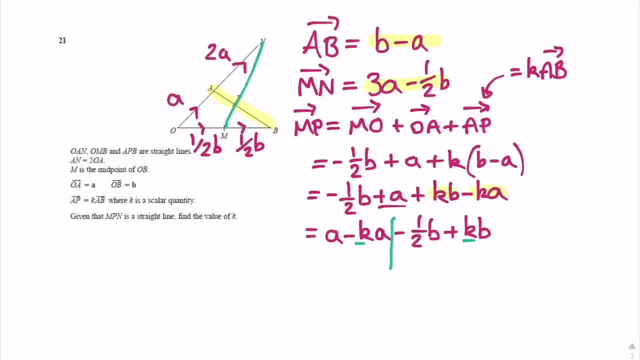 factorize this in steps. i'm just going to separate this with a little line. i'm going to factorize the a's and then factorize the b's. so if i factorize a out, at the moment we have a brackets one, one minus k. just factorizing the a out there and on the right hand side here, just to make sure that. 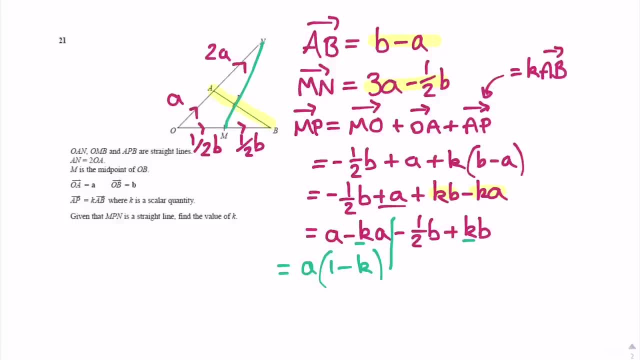 we've got a matching symbol at the front in the middle here, just like we have over in our mn. i'm just going to- let's just circle that this one here. we've got a minus half b up there. so to ensure i get that, i'm going to factorize out minus b. so i'm going to factorize out minus b and if we factorize, 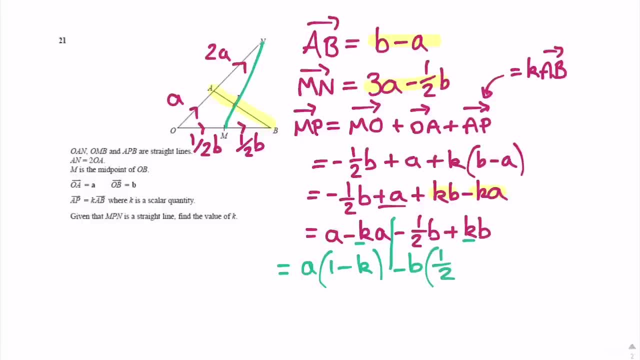 out minus b, we get a positive a half here, so a half, and then factoring out, factorizing minus b, a positive kb would give us minus k, and again, there are other ways of doing this, but this obviously just matches the a minus b just up there. so at the moment our coefficient of a is one minus k and our coefficient of b there is a half. 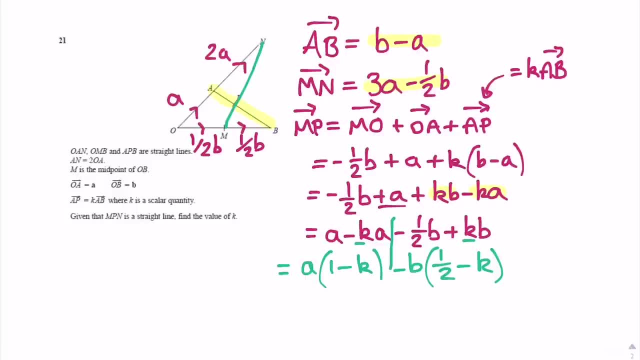 minus k. now we've already said: i'm going to write this down, the coefficient. let's write this down: coefficient. there we go. coefficient of a must be six times greater than the coefficient of b. there we go. okay, got that in there. so coefficient of a must be six times greater than the coefficient of b. 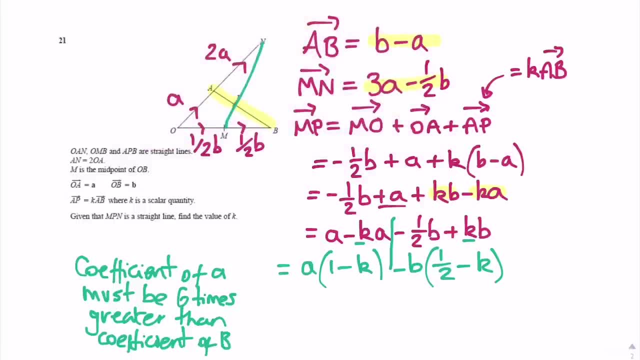 now, if we look at actually how to apply that in terms of a little equation here, we can say, okay, well, a this one here, one minus k. so one minus k has to be equal to six lots of this one here. so six lots of a half minus k. 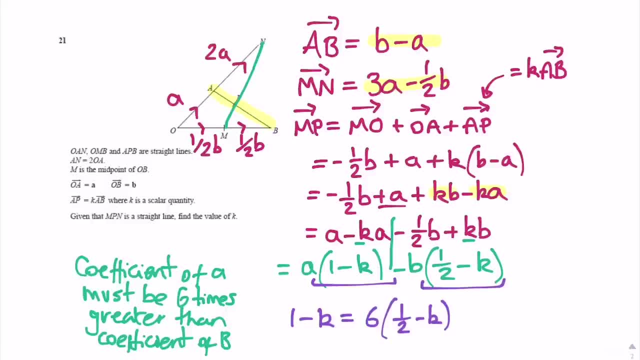 there we go. and if we expand that bracket, so multiplying it by 6, let's see what we get. so we get: 1 minus k equals 6 times a half is 3, and 6 times k equals 6k, so minus 6k. 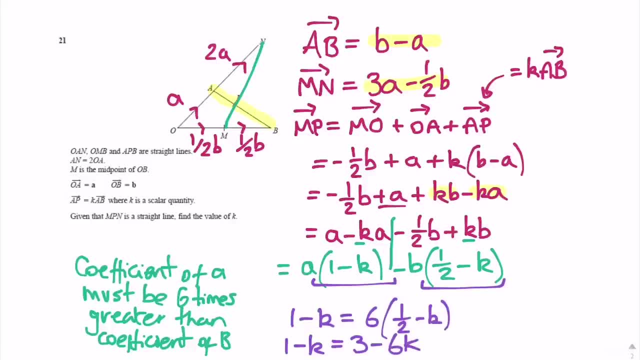 i'm gonna write that a bit clearer than my k there. okay, so now we've just got like a nice simple equation that we need to solve. so if we just go about actually solving this equation- i'm going to bring this up slightly just to here- let's actually solve that. so. let's add 6k to both sides, um, and what do we get when we do that? we get an而且abwaard rag seen as denotationomanious to that. so let's add six k to a half minus k, and and see how much property we have to solve this. i'm gonna bring this up slightly just here. let's actually solve that. so let's add six k to both sides, um, and what do we get when we do that? 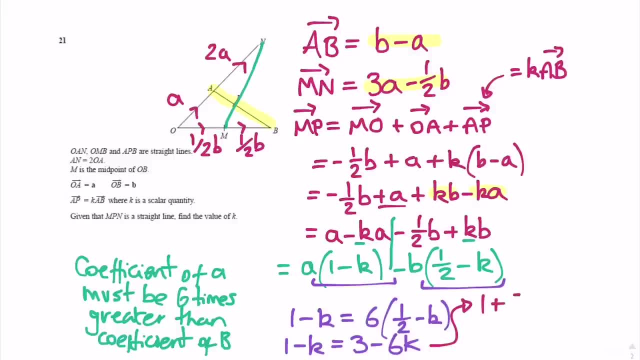 we get when we do that? we get 1 plus 5k equals 3, take away that 1, gives us 5k equals 2, and then divide by 5, we get k equals 2 over 5, 2 fifths. and there we go. that is our. 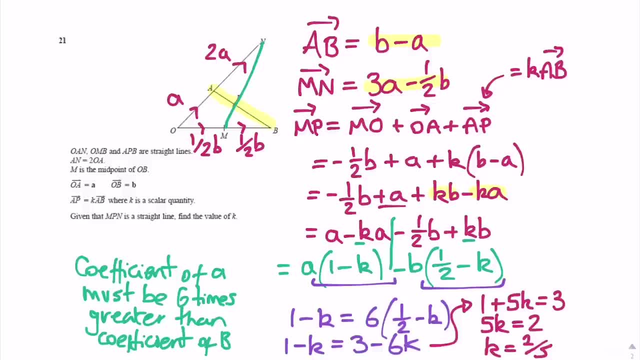 value of k there 2 fifths, and actually that's answered the question. So there we go. our value of k is 2 fifths. just following that little bit of an approach, just comparing the coefficients there on part of the line and making sure that they match obviously. 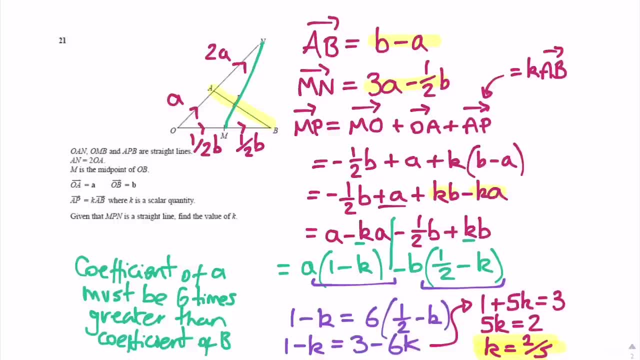 that proves that lines are going in the same direction when they've got that matching vector. So there we go. that's just a way of doing this question. Again, I think there are probably lots of different ways of doing that question. it is quite a complicated one. 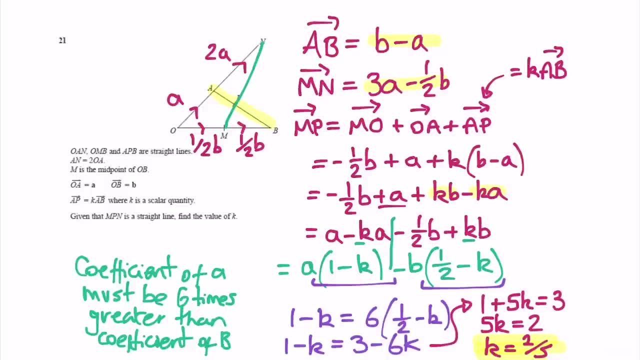 where the methodology, especially in mark schemes here, was left quite open. there was no specific way of answering it given in the mark scheme. but that's just one way that I looked at this question and thought about how to solve it in that different approach. 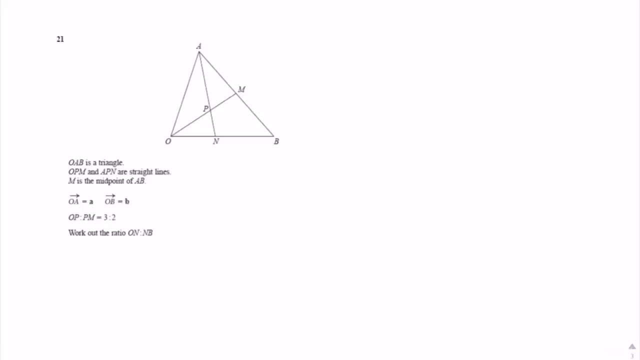 there. Okay, we'll go and look at another question now. Okay, so moving on to this question then. Now it says we've got some straight lines there that we can see Again. it says m is the midpoint of a to b. Now it says o to a. let's have a look, that's. 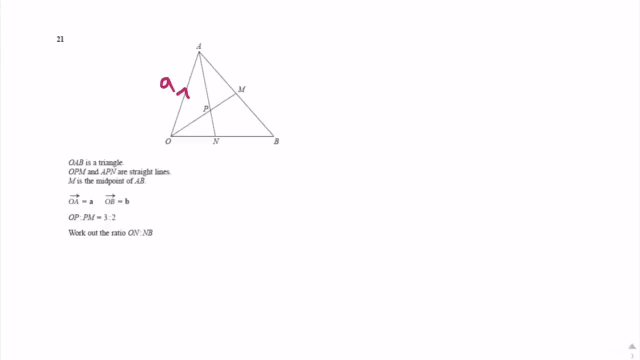 this one up here is a, and o to b is b, But it doesn't tell us how far onto that line that n is. so I'm just going to write that as b. there we go Now. it does say m is the. 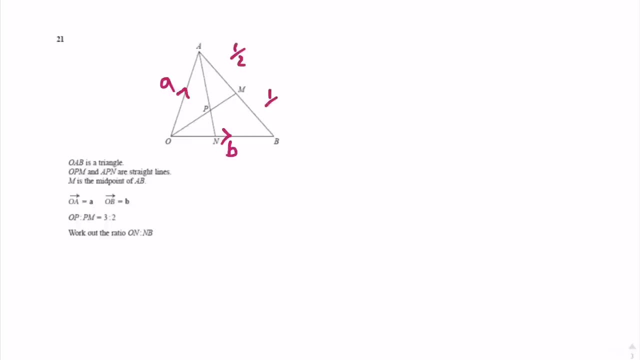 midpoint. so just in case you don't want to forget that, just put half and half here, just so we can see what's going on. Now it says: find the ratio o to p, p to m. So again we're going to have a look at some of the lines here and probably having to think about maybe 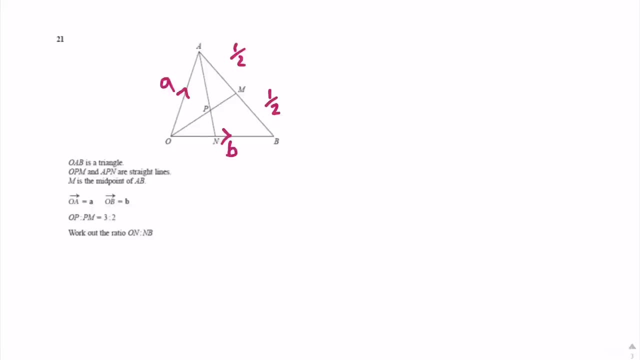 coefficients, again like the last question. but let's have a little look Now to get from a to b that line at the moment, because obviously once we can get from a to b we can get from a to m, and once we can get from a to m we can get from o to m. So I think that's the 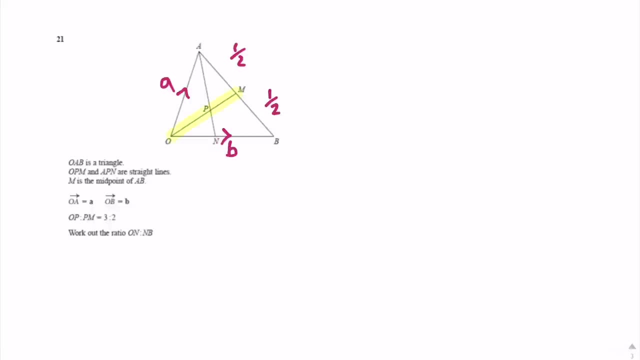 little journey I'm going to go on. at the moment I want to have a look. well, how do I get from o to m? And to do that, I go from o to a and then down from a to m. Okay, so to. 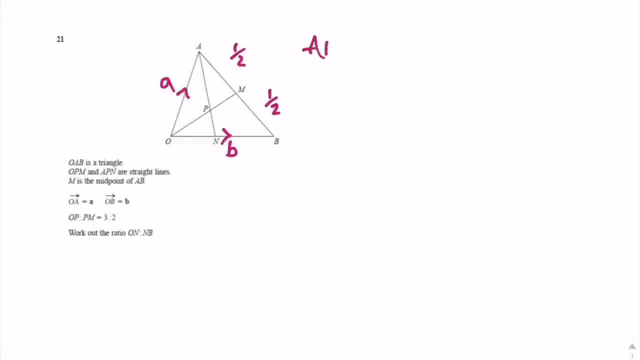 do that. first I need to find the vector a to b. So a to b is b minus a. Let's have a look. or if you do it in the order, it's minus a plus b. So for minimum amount of symbols there. so we have b minus a Now to get from a to m. 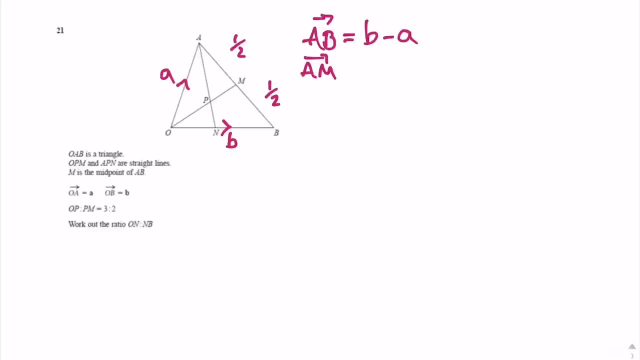 it's going to be half of that, so a to m. So a to m is half of that. I'm not going to open the bracket, I'm just going to do half b minus half a Save. so opening the bracket and doing a little bit more working out for the moment. And now let's have a look at o. 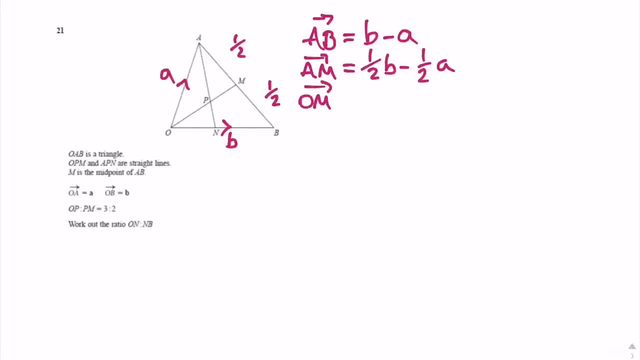 to m, So o to m following that same route, so I'm going to go down from a to m, so I'm going to go from o to a, so I'm going to add in an extra a. So obviously, at the moment, 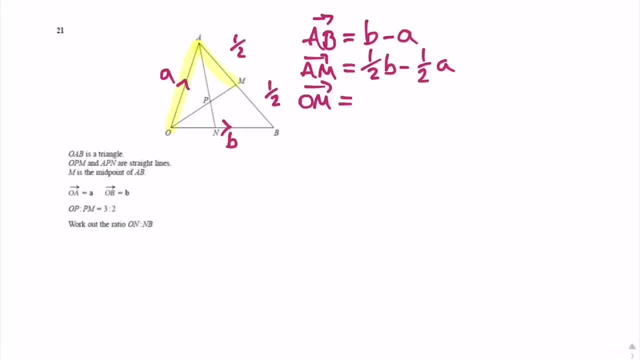 let's have a look. we're going up an extra a now, Moving down this half of that vector that I've just found. So from o to a is a plus half b minus half a, that vector above there, And let's tidy that up- a minus a half a is. 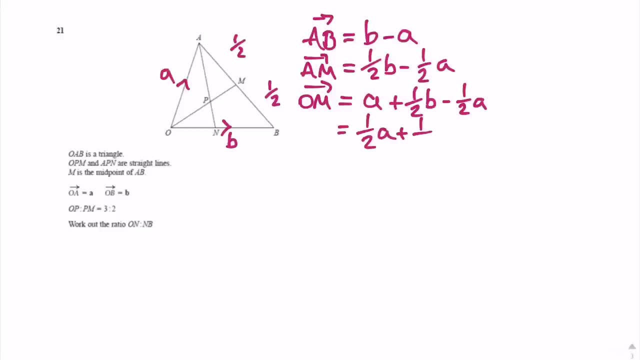 a half a, so we have a half a plus a half b. There we go, and that's our vector: o to m. Now let's have a look at something slightly different. What about getting from a to p? Okay, moving down this line that we're actually looking at in the question, because we want 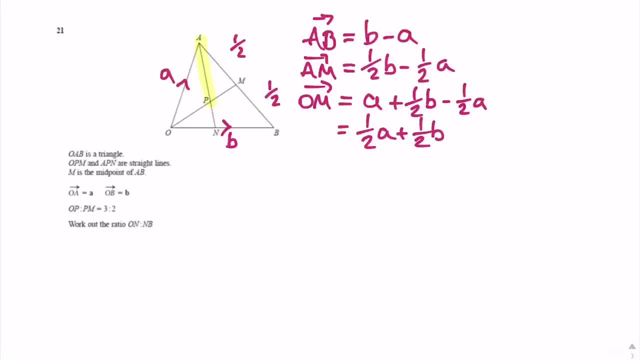 to have a look at o to p. So what about getting down here From a to p or p to a to n or something like that? Let's have a think about how we can do that. So a to p at the moment: what do we actually have? How can we actually get? 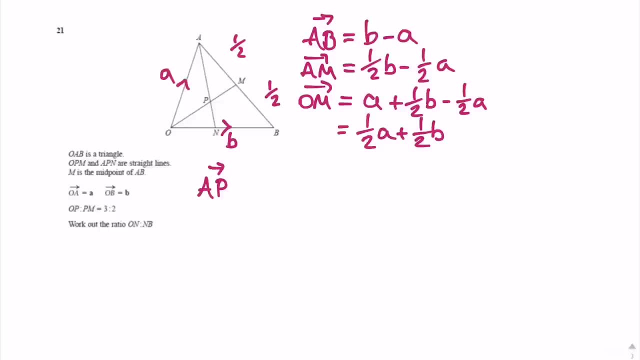 to there. So we can do minus a, we can go down here and then we can go part of this line o to m. Okay, it says that o to p, p to m is in the ratio three to two down here in the information. So let's have a look at putting that information on there. So that's. 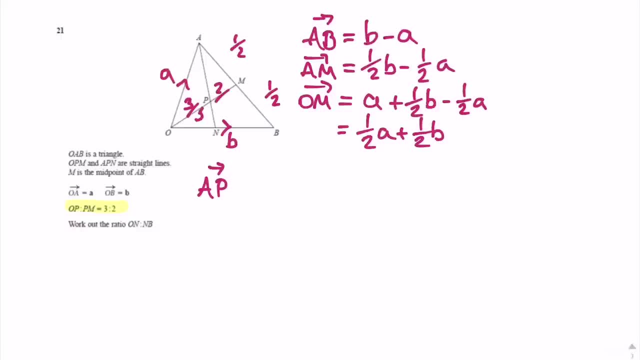 a five. so that's three fifths of the line there and two fifths of the line there. So in order to get from o to p I would have to do three fifths of o to m, and we've just found o to m, it's up here. so three fifths of that. So to get from a to p, we'll first. 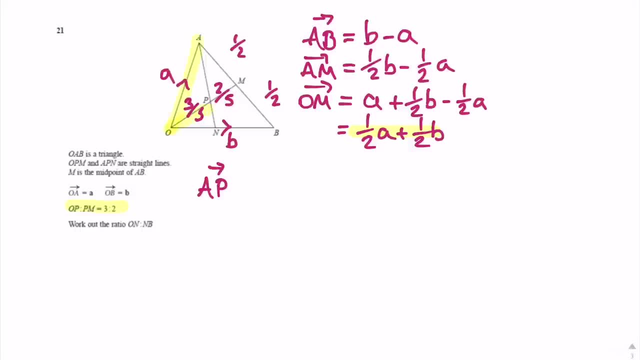 move down minus a and then three fifths of o to m. So let's have a look. So from a to o gets us minus a, and then we're going to add to that three fifths of that vector above there, which is a half b plus a half a, or a half a plus half b, half a plus half b There. 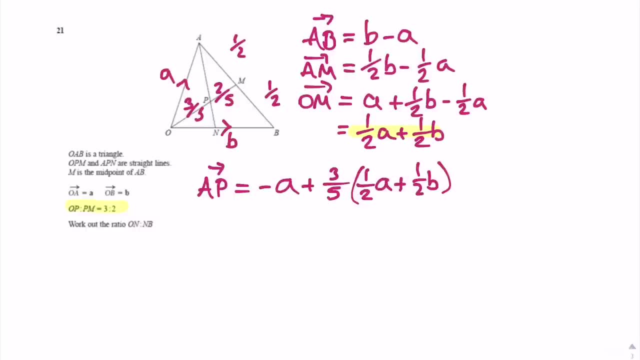 we go And then we just need to expand that bracket out. So what do we get there? We get minus a plus normal fraction, rules times in the top, times in the bottom. So three tenths a plus three tenths b. There we go Right. at this point it kind of looks like. 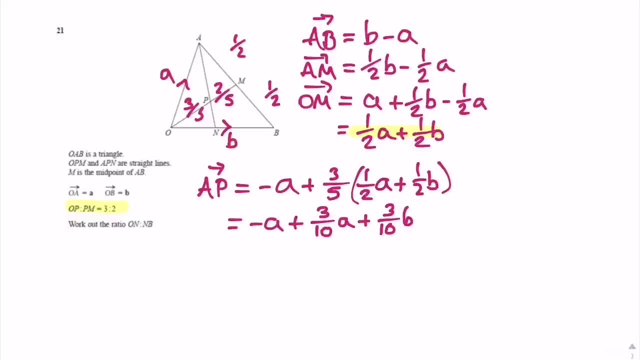 what on earth are we actually going to do here Now? let's just simplify that down. So we've got minus one a plus three tenths a. So that's minus ten tenths plus three tenths, which is going to seem a little bit weird to do, but that's going to give us minus seven. 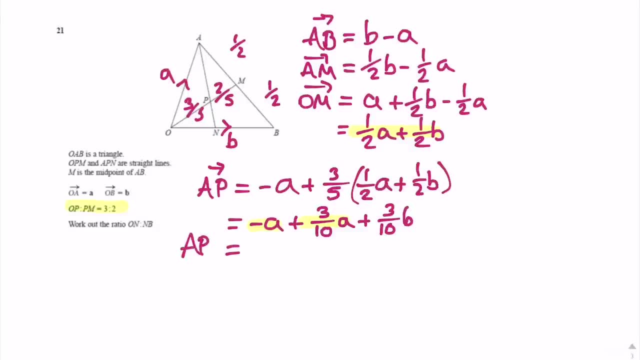 tenths- So that's a to p when we tidy this up- actually gives us let's have a think, let's do the b's to start with. So we've got three tenths b's that aren't going to change. 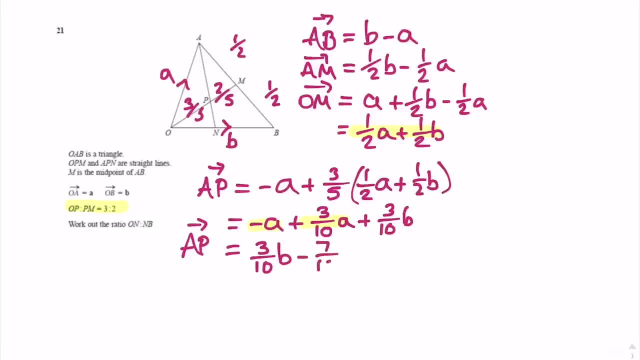 and then we've got minus seven tenths a- Okay. minus one a plus three tenths- Okay. there we go. Now we can actually factorise that. Obviously, a lot of the times you can factorise these, We could take one tenth out. There we go. we'll see if it helps us. But if we take a, 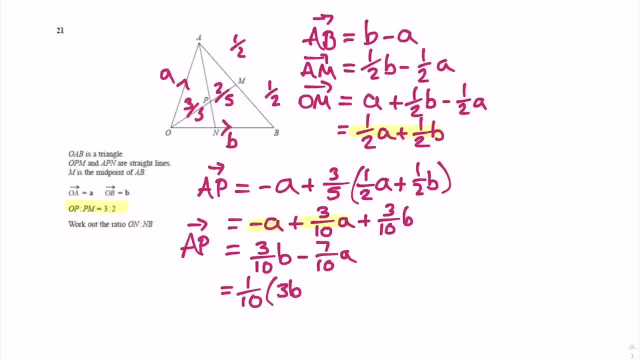 tenth out, we get three b minus seven a. Now that may not help us there, but at least we've got that vector a to p there. Now let's see if we can have a look at comparing these coefficients then with the other one. Now, if we have a look at the line a to n, we've just got the 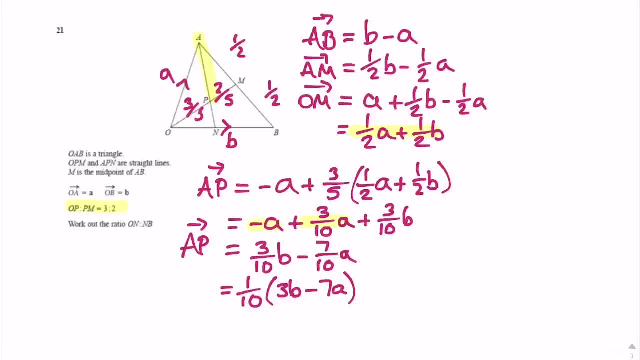 line a to p there. Okay, that line a to p is one tenth three b minus seven a. Now, if we have a look at the full length of the line a to n and see what we actually get for that. So a to n, let's have a think. a to n. 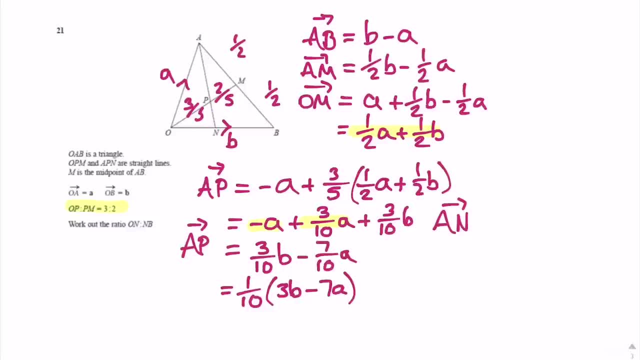 actually gives us the vector there. Let's have a look: a to n is minus a, moving down from a to o, so minus a. And then we're going to add k, lots of b. We don't know how much that is there. 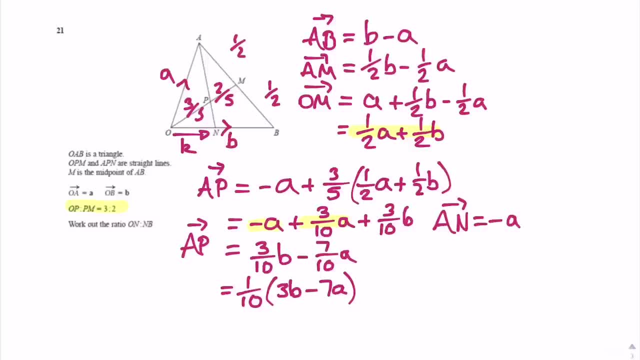 so let's just think of this bit here as an unknown. We've been using k in the other question, so let's go for k. So plus k, lots of b. Okay, that's not a k. I'm going to have to do my k differently. Here we go k, lots of. 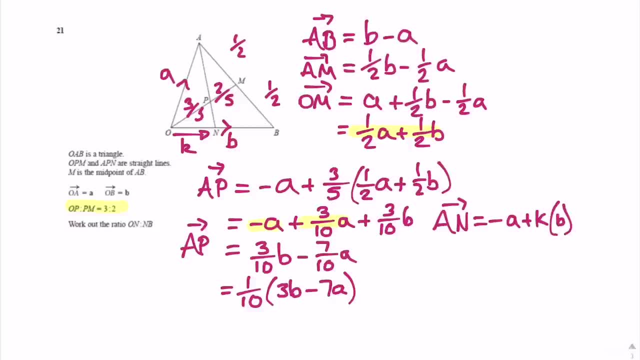 I'll just put b in a bracket there. So it's minus a, plus k, lots of b. Now let's have a think. So a to n is what we're looking at at the moment, and a to n is an amount, or it's a multiple of a to p. Okay, we'd have to times a to p by something. 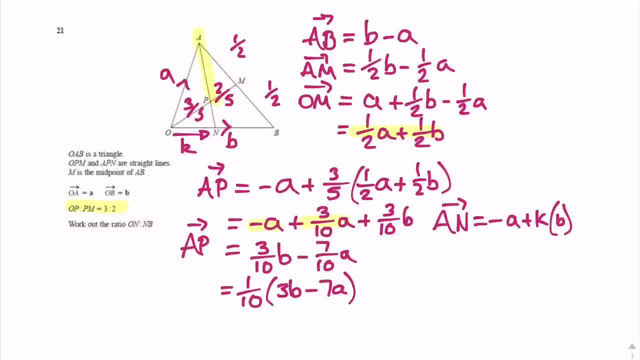 to get the full length there. So a to p, we've already found, and to get from a to n it'd be a you know a bigger amount of a to p. So let's just write that in terms of you know, a to p. 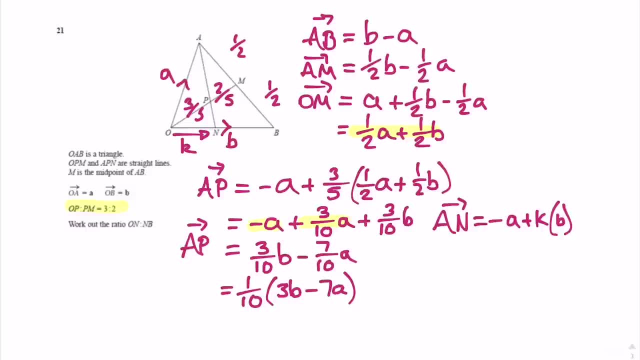 So let's just write that in terms of a to p. So let's just write that in terms of a to p. So let's just write that in terms of a little vector here: x, lots of a to p or an amount of. 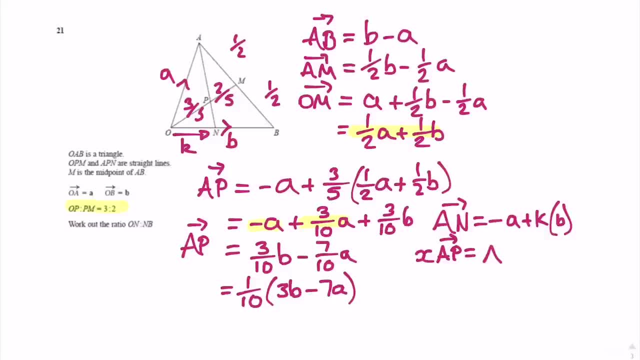 a to p there is going to equal the same as a to n. Okay, we're going to figure out how much that actually is and see if we can figure that out. So a to p, we've just worked out. it's that one. let's highlight it. it's this vector down here And we're going to times that. 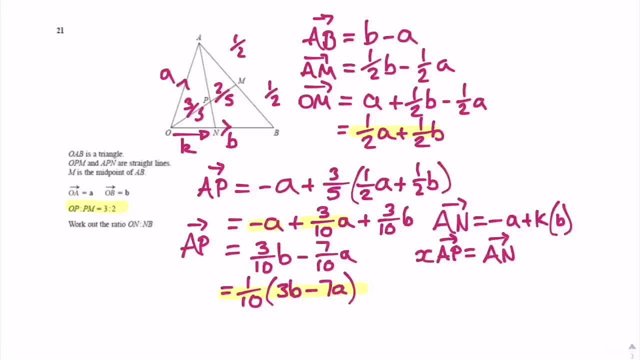 by some multiple, which we're going to say is x. We don't actually know what that is, so let's times that by x. Now, if we multiply that by x, so one tenth times x gives us one tenth x or x over 10.. So we can say it's x over 10, lots of 3b minus 7a. 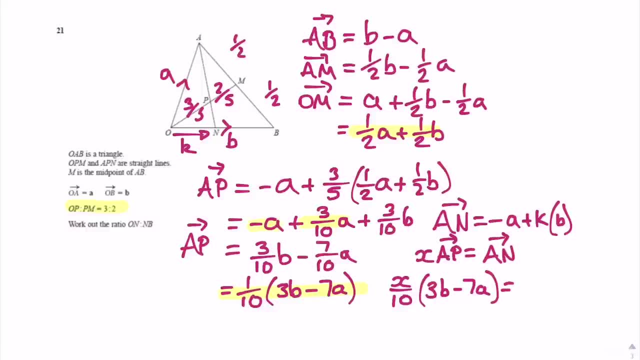 And that has to be equal to that little vector above there, minus a, plus k, lots of b. There we go Right. so what have we actually got here? We've got some coefficients that we can actually have a look at now. So at this point, this is where the question really starts to step. 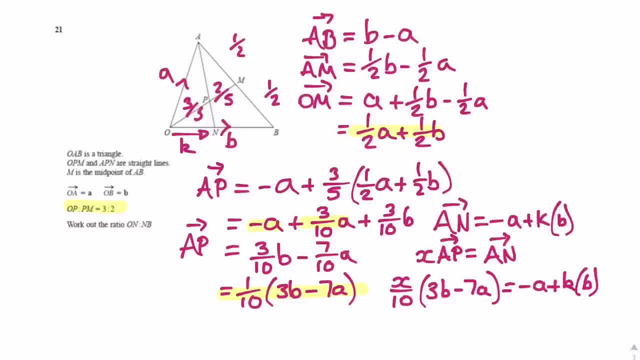 up and we've got some tricky stuff here. Now, if we have a look, if we expand this bracket out, this one here, so timesing this by the x over 10, we get 3x over 10b minus 7x over 10a. 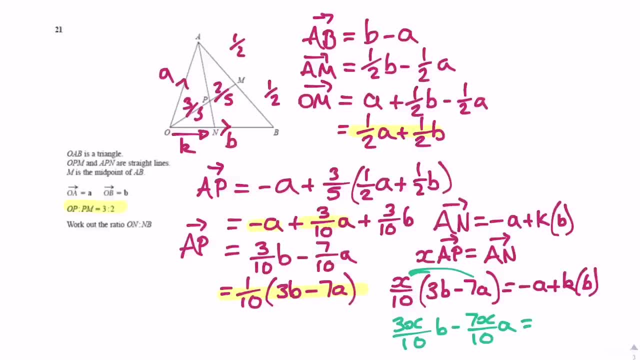 And if we actually look at comparing the coefficients now, because it says that has to equal minus a, plus k, lots of b. Once we start to compare the coefficients we actually do start to get some equations here. Now, the coefficient of b is: 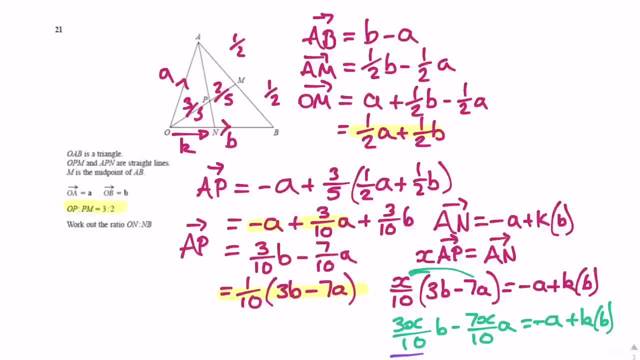 apparently in this part, 3x over 10, and over here it's k. So if we write that as a little equation, over here we've got 3x over 10, and that has to equal k, whatever that is, So that 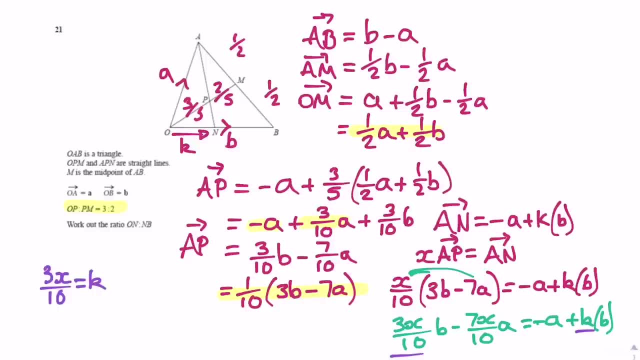 gives us a little equation that we can have a look at. And then if we look at the a's, we've got minus 7x over 10 equals the coefficient of a there, which is minus 1.. So let's write that as another equation. So we've got minus 7x over 10. 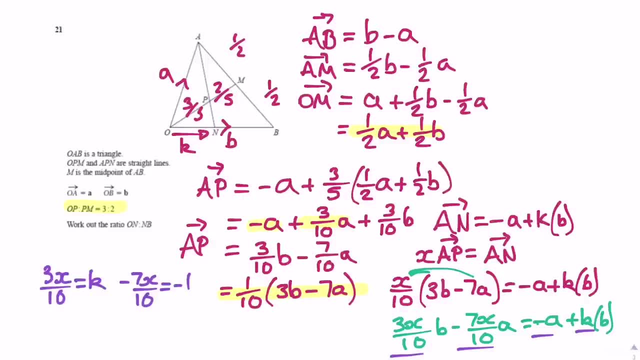 minus 1.. Now let's have a look at just solving these. So that one on the left there, if we times by 10, we get 3x equals 10k, And divide by 3, we get x equals 10k over 3.. Solving the one on the. 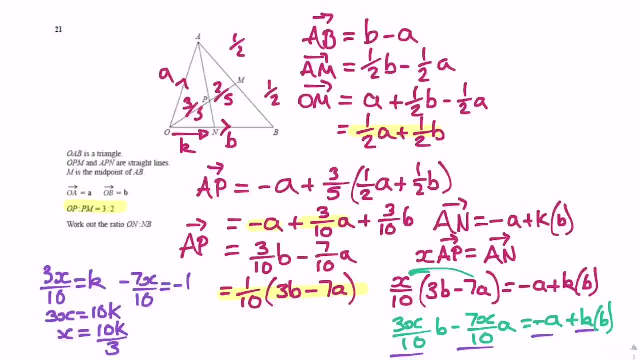 right, they're both negative there, so we can cancel out the negatives. We can times by 10, we can just get 7x equals 10.. And there x equals 10 over 7.. So now we have two equations that both equal x, So we can say that they both equal each other. 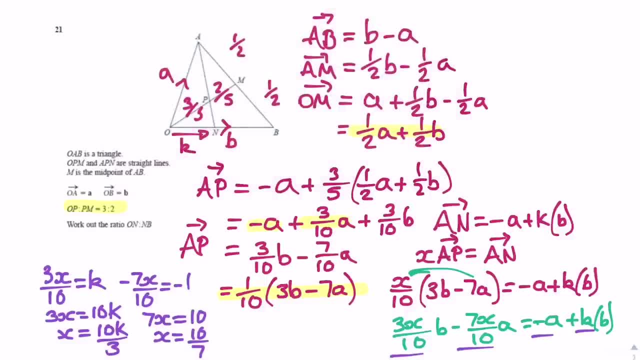 And if we set them both equal to each other, let's see what we get here. So we've got 10k over 3. 10k over 3 equals 10 over 7. And then we can cross, multiply that, or actually no. 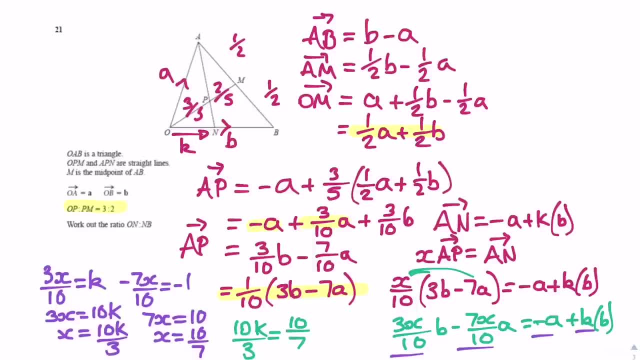 let's not do that. Let's split this fraction up. Instead of doing it that way, let's split this fraction up. So, rather than saying 10k over 3, I don't want to get rid of all of that- let's just say it's 10 thirds k. 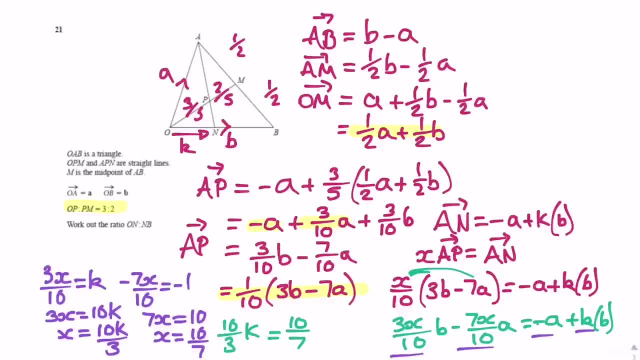 So keeping the k separate from the fraction 10 thirds k. It's a little bit quicker here. actually We can just divide both sides by 10 thirds, And dividing by 10 thirds look, is the same as timesing by 3 over 10.. So k equals 10 over 7 divided by 10 thirds. 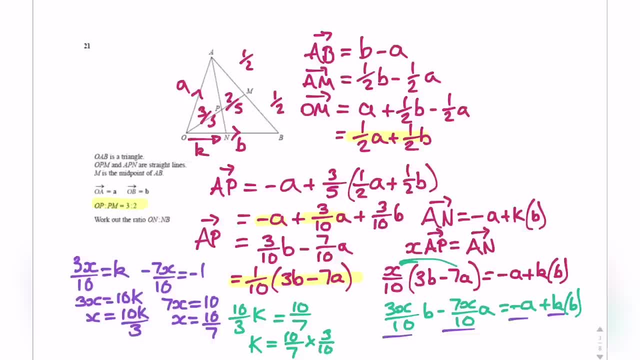 which is the same as timesing by 3 over 10.. And that gets us 30 over 70,, which is 3 over 7, if you simplify it or cross simplify there, Let's have a look So we can cancel off the 10s. look. 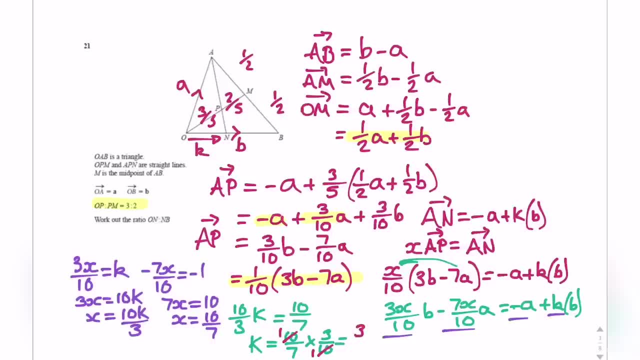 They become 1.. So it's 1 times 3 on the top, which is 3.. And 7 times 1 on the bottom, which is 7.. So we get the answer 3 sevenths. Now, what does that actually mean in terms of this question? 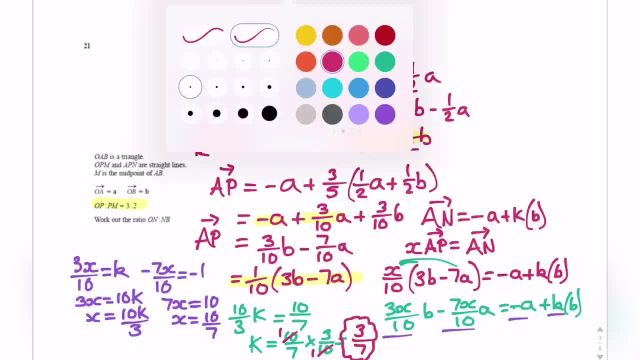 So all of that was to find. I almost get lost with the working out when you start to do these. That was o to n. So o to n is the k. Obviously, here it is. This is the k that I was talking about. 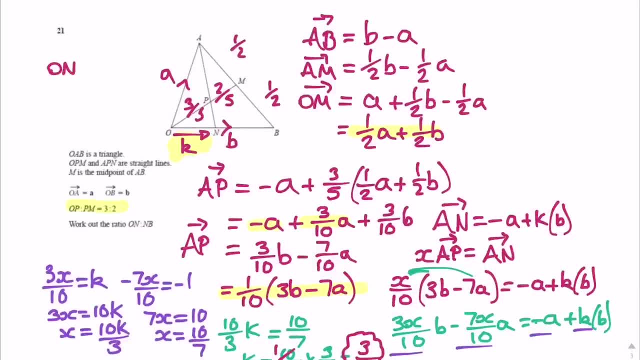 So o to n- let's write that down- was 3 sevenths, that value of k, Which means that n to b is got to be 4 sevenths. There we go And remember. the whole question was asking us to work out the ratio o to n, n to b. 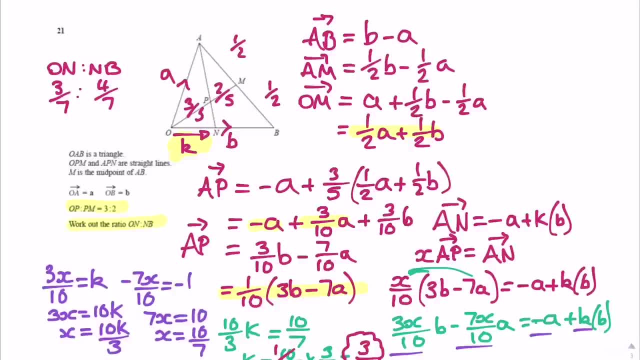 So that is the ratio just up there: 3 sevenths to 4 sevenths. obviously, times both of those by 7 to get them as whole numbers And we get the answer 3 to 4.. There we go And that is our actual final answer. there I think, Yeah, that is what it wanted. 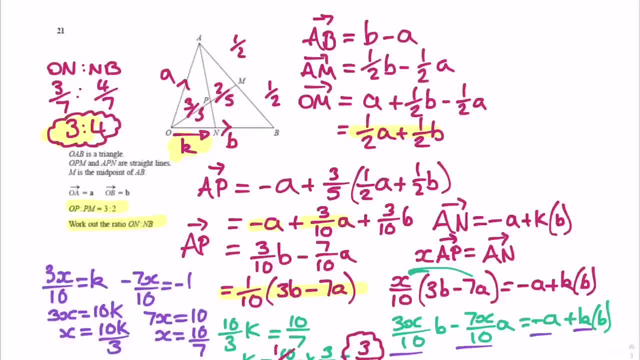 It wanted o to n, n to b. So there we go. There's our final answer for this question 3 to 4.. Obviously, with a question like this, we're going to have to do it again. So we're going to have to do it again. 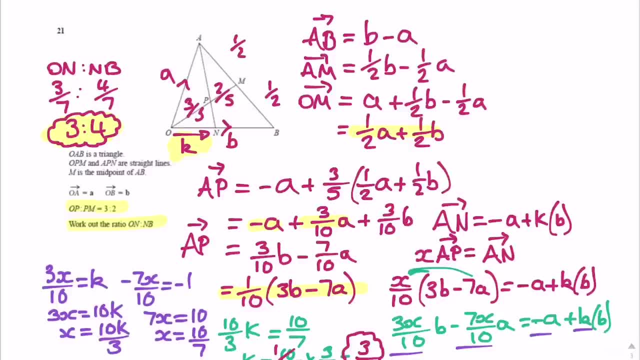 this is. you know it's pretty mad question, but there's a lot of marks to be picked up before all those last steps. so I think as you get to this part here, you basically got all the marks bar the one mark there, for all that working out at the end okay. so it's a massive question, but 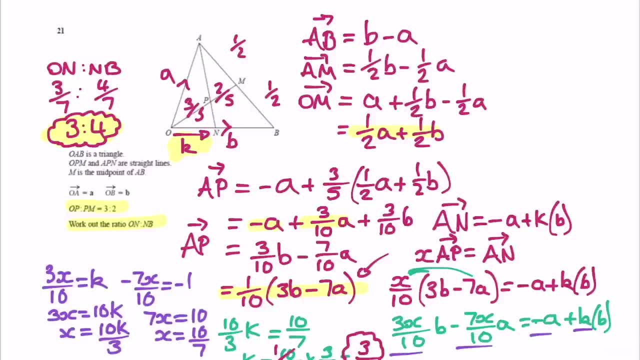 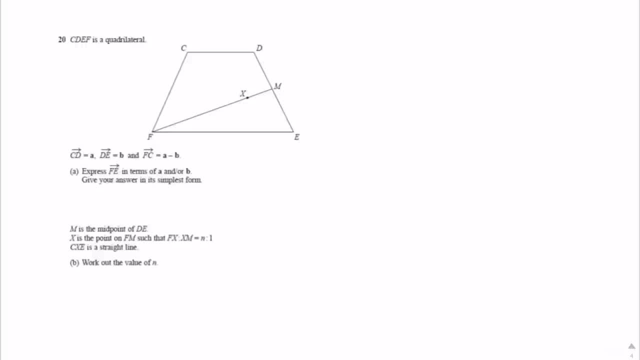 there you are. that's how. that's one way of getting the answer to that particular question. let's have a look at another one. okay, so this question says we've got two steps. so the first step is asking, asking this to do, and let's just get some information on the diagram. first. it says c to d. 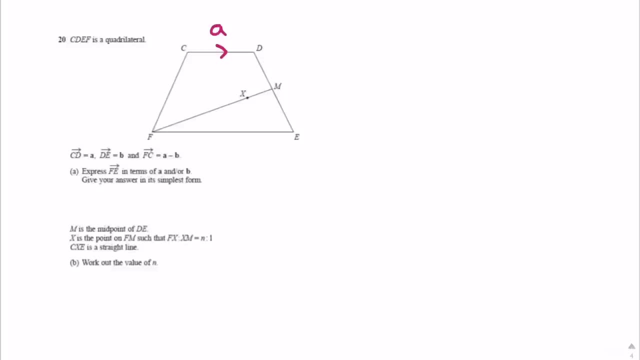 equals a, so that's a. it says d to e equals b and it says m is the midpoint there later on in the question. so let's have a look, let's just write that in. there we are. so that's going to be half b and that's going to be half b as well. there we are. and then it says f to c is a minus b. 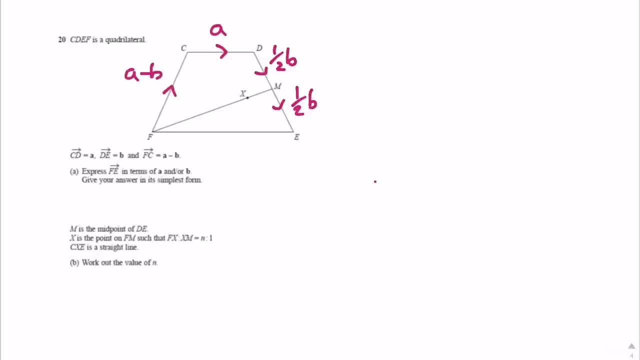 so that's a minus b. there we go right. so it says express f to e in terms of a and b. so f to e, we would have to go up to c, across to d and down to e. so it's basically just adding all those vectors together. and if we add them all together, let's see what we get. we get a minus b. 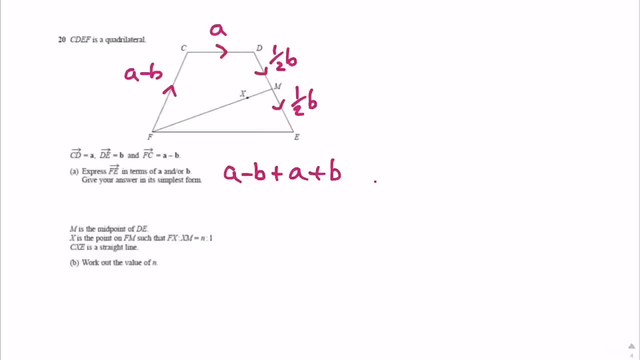 add a, add b, and if we join that all up, look, you've got two a's and the b's cancel each other out. so the answer is just two a there. so there's our little vector, and that is the vector f to e. now, normally when you're given a part a here, it normally does link into part b. so I'm going to 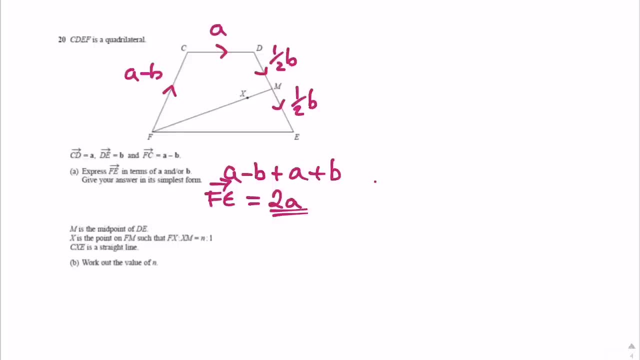 label that and see if we want to use that later. we may not need to, though, but we'll have a look now. it says m is the midpoint. we've already put that on- and then it says x is the point on fm, such that f to x, f, x to m is in the ratio n to one. okay, so that is that ratio there. that 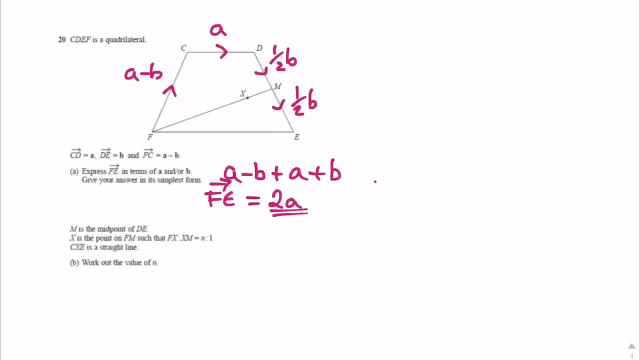 we've got for that. so f to m, f to x is n and x to m is one right, and it wants us to work out the value of n, like my. my one there almost looks like a two. I'm going to get rid of that and just put a. 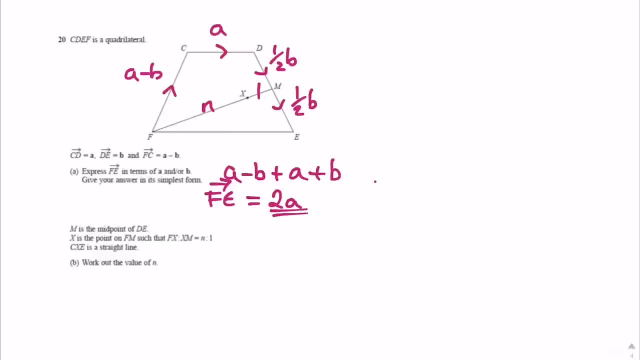 nice easy one. in there we go and it says c, x, e is a straight line. let's draw that in a different color: c to x, to e. there we go, right. so work out the value of n now. a couple of different ways that we can approach this, but ultimately we're going to have to work. 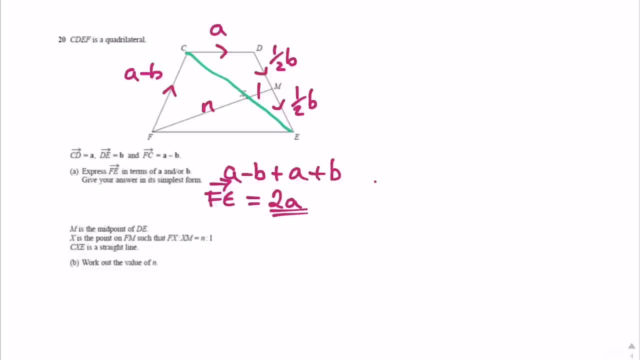 out this line f to m. that's the unknown line in this question. so we want to know what the full length of this line is. once we know the full length of that line in terms of these vectors, we can sort of go about looking at this question in a slightly different way. so let's have a look. 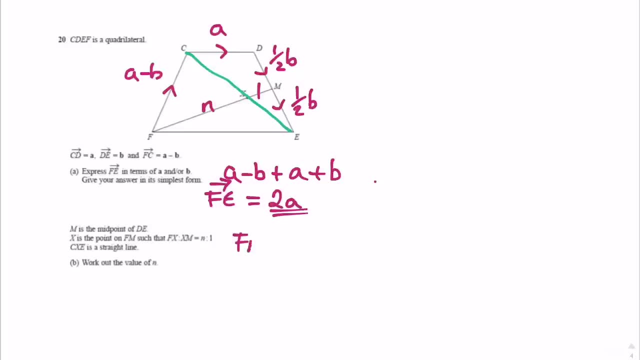 now to get from f to m. what have we got to do there? so from f to n we have to go a minus b, moving from f to c, plus the a to get us across to d, and then plus the half b. sorry, that should say a, not c. 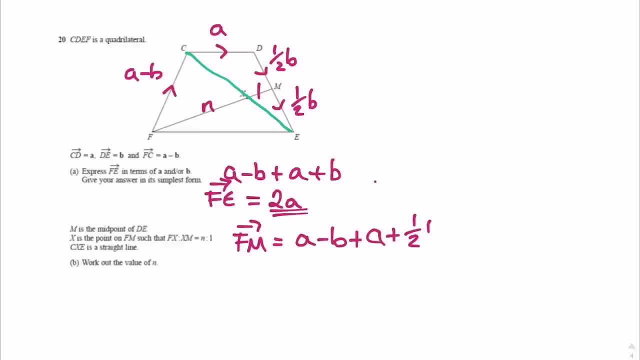 from c to d is plus a, and then plus the half b to get from d down to m. simplifying that all down we've got two a's and then minus b. plus half b is minus a, half b and that is our vector. f to m. 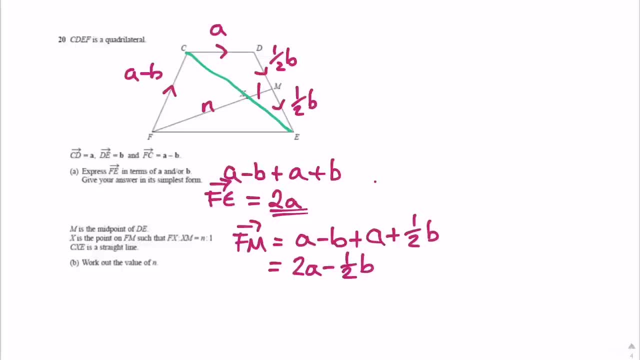 there. now let's have another thing. so what about just going part way along that line? now we don't know what the amount of the line is, but we don't know what the amount of the line is, but we don't. we know it's in the ratio, we know the ratio is n there. so if we have a look at actually working, 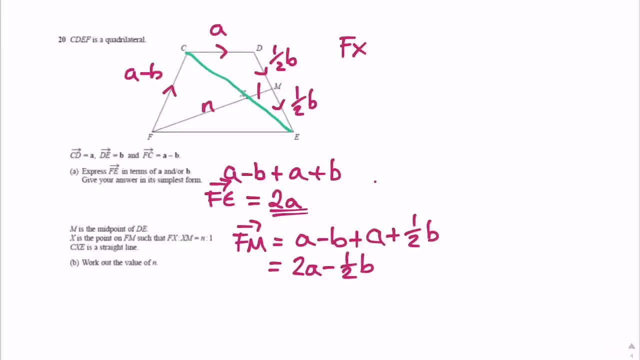 that out. let's bring it up to the top to get from f to x. it's going to be n lots of whatever that ratio is, n lots of the vector we've just worked out. so n lots of two a minus half b, so n lots of. 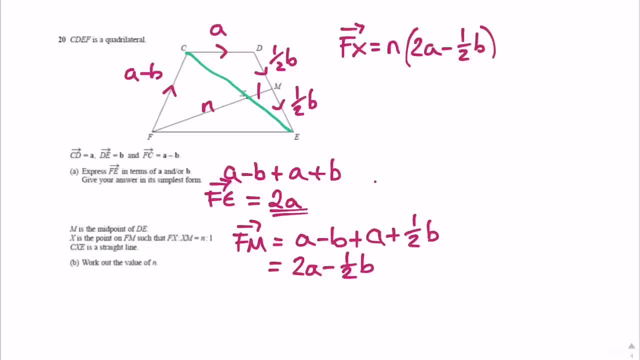 two a minus half b- there we go. let's write that down and let's expand that out. so we get two a n minus half b n there we go. n lots of that full line. now obviously we don't know what n is, but we can have a look at how we can work this out in a sec. 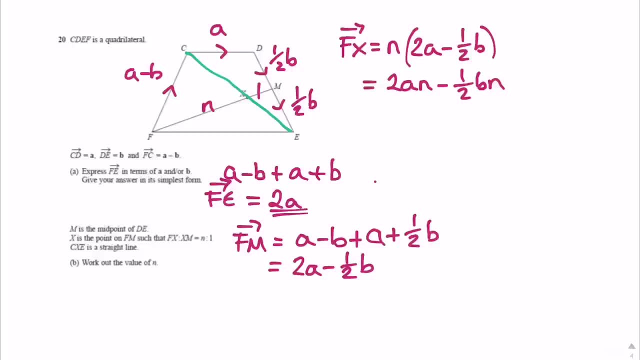 because we can have a look at this other vector, c to x and c to e, and have a little think about those. so to get from c to x i would have to do c to f and then i would have to do f to x, which again we've just written, just written down just there. so let's write that down: from c to x. 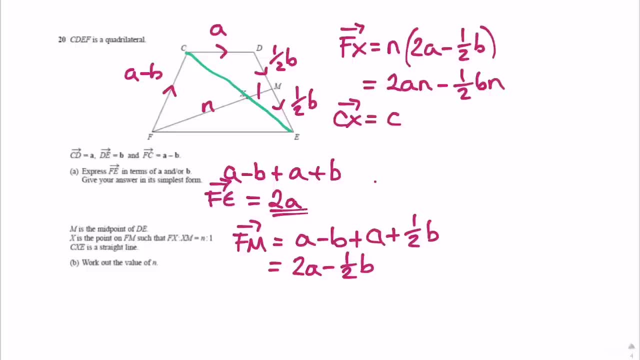 i would have to do c to f, add f to x. there we go. so writing these down, let's see, c to f is uh, moving backwards through a minus b. so i have to reverse the signs there. so we've got minus a plus b, and then we're going to add to that the little. 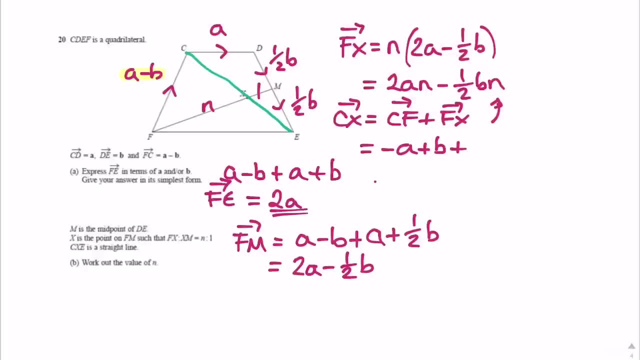 vector that we've just worked out, this one just here. so plus two a n, minus half b n. and if we simplify that all down, let's have a look, let's join up the a's. so if we join the a pieces together and the b parts, we have plus b minus half b n. 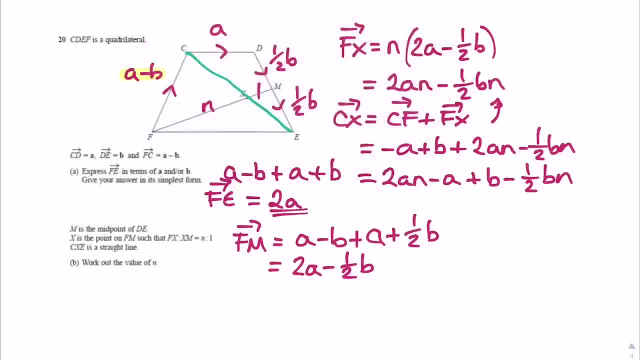 right. so c to x, there our little vector, we can actually factorize this. so if i factorize the a pieces there, take out the factors of a, because we're going to have a look at some of these coefficients here. i'm going to bring it down here. so we have a lots of two n minus one when we 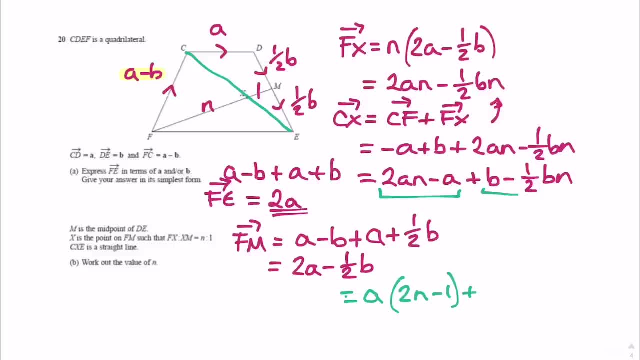 factorize that, add and then factorize the b's out here. b lots of What is it? 1 minus 1 half n. There we go, So that is our vector c to x. Now, the whole reason we've actually looked at this vector c to x is because it has to match one of our other vectors. 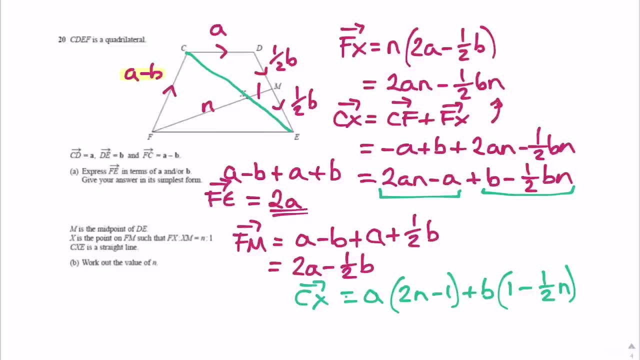 And I've just completely lost where that vector is: c to e. Now, c to e is the full length of the line. So the full length of the line there, c to e, we can actually find the vector for, So to get from c to e, if we write that over here, because this is the one we're going to compare: c to e. 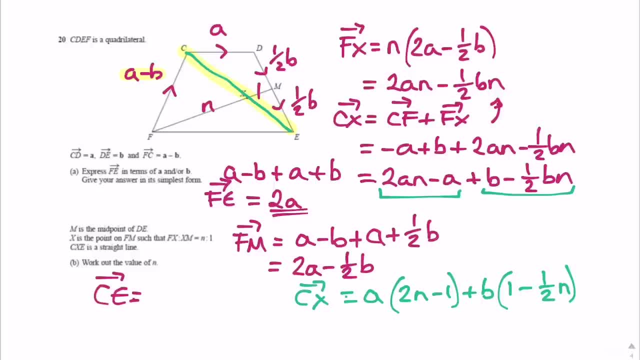 that is the vector. So I think you go along a down b, so it's a plus b. There we go. So if we have a look at the coefficients here, because they have to match, obviously it's going to be a different multiple, but the coefficients of a and b have to be the same. 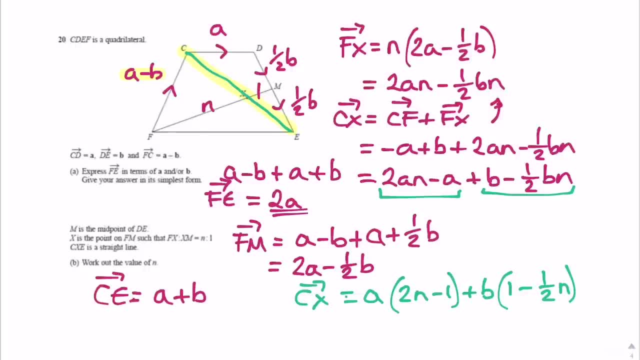 if it's the same straight line which it says in the question. So, in order to match the coefficients, look the coefficient of a and the coefficient of b, and we can treat this in a different way to one of the previous ones because the coefficients are the same. 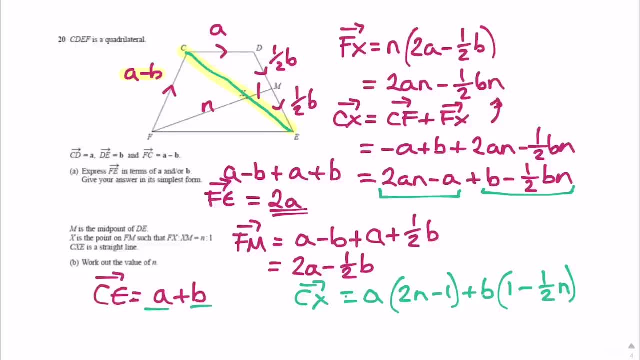 We don't have to think of one being bigger than the other or a certain amount bigger than the other. We can just say that they're actually going to be equal. Okay, so, because the coefficients are equal for a and b, all we can say is: 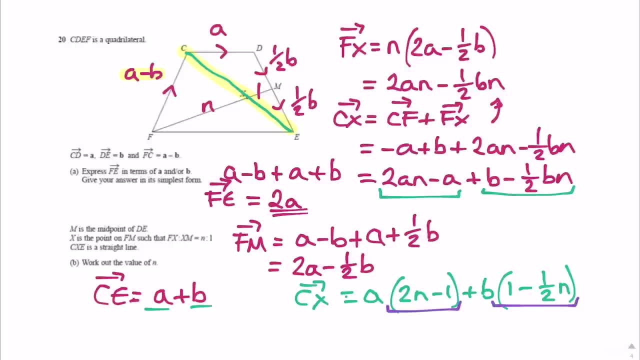 we can just say that this coefficient of a has to be equal to this coefficient of b. Okay, so if we set them equal to each other, we can say 2n minus 1 has to equal 1 minus a half n. There we go and we can just solve that equation. 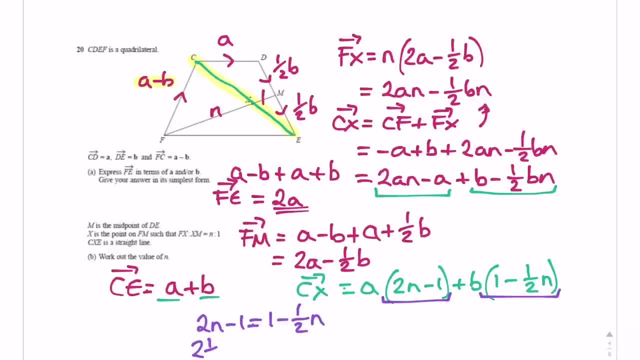 So add a half n to both sides. 2 and a half n minus 1 equals 1.. Add the 1 to the other side, so let's bring that up here. So 2 and a half n equals 2.. And then we're going to have to divide both sides by 2 and a half. 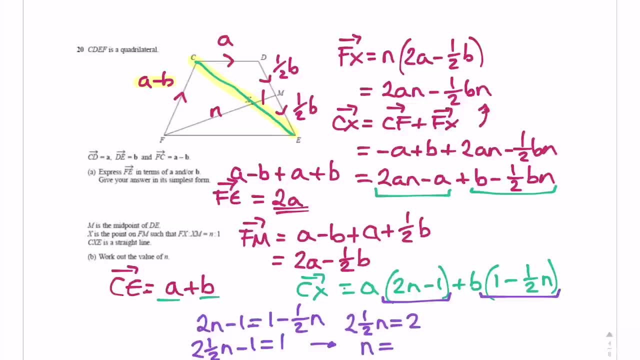 So n equals- and don't forget, 2 and a half is the same as 5 over 2.. So we're going to divide by 5 over 2, which is the same as timesing by 2 fifths. So it's 2 times 2 fifths. 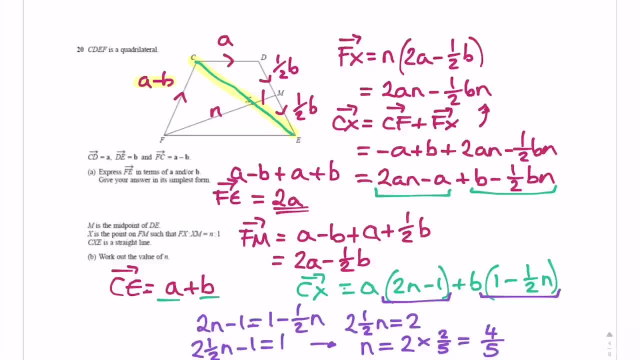 And 2 times 2 fifths is 4 fifths. There we go, so 4 fifths. So n over, there is 4 fifths, which means that one part is 1 fifth. Okay, so it's 4 fifths of the way along the line, and the other part is 1 fifth of the way along the line. 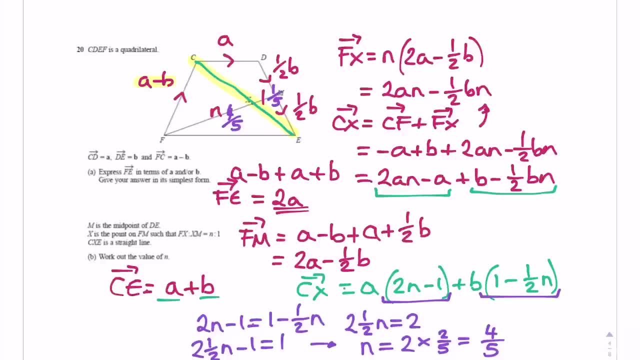 So, as a ratio f to x, x to n, which is obviously written to us in the question here, that ratio would be- let's do this over here- 4 fifths to 1.. And again it wants it in the ratio n to 1.. 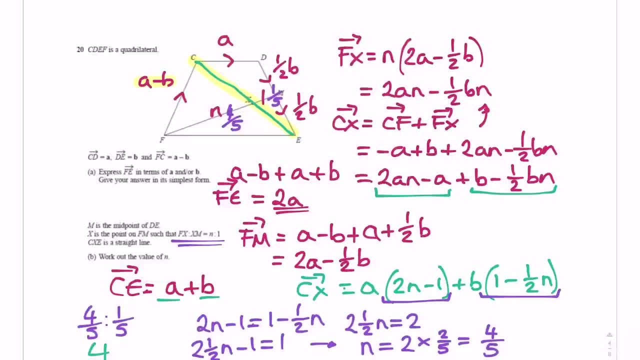 So timesing both of those by 5 gives us the ratio 4 to 1.. Okay, so that's our ratio there, 4 to 1.. And that obviously gives us our value of k as being 4.. So our final answer there, sorry. value of n. 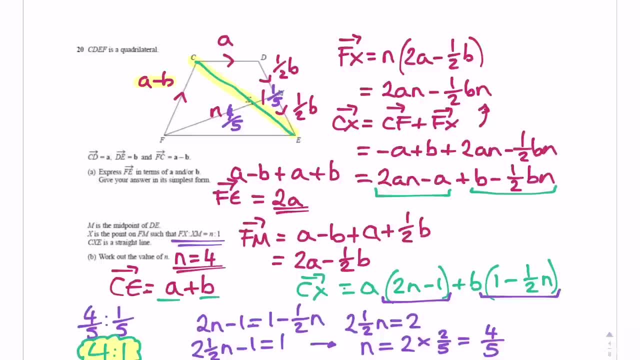 So n equals 4.. There we go and there's our final answer. Again, another quite tricky question there. But there you go. that's a little process of how to work that out. Obviously not a huge amount. I've got a lot of explanation here on actually how to work them out. 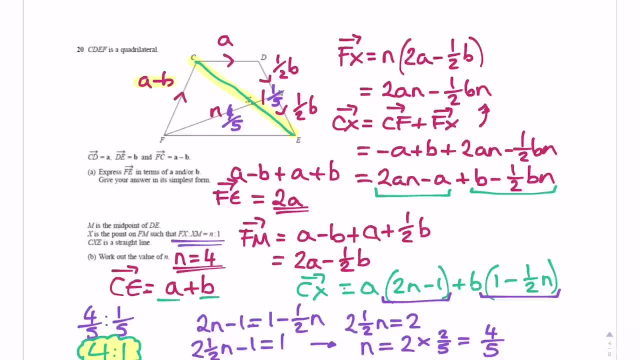 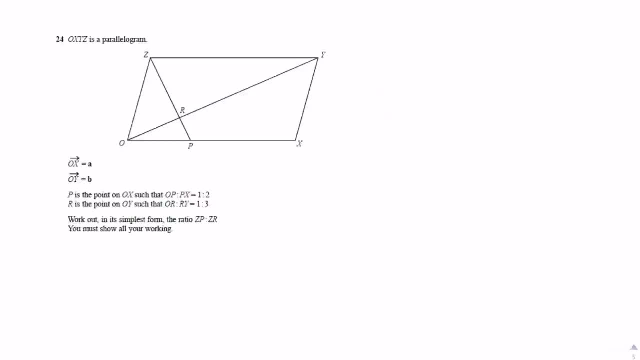 But obviously just think about a process to actually get towards the final answer here. Okay, moving on to the next question. Okay, so the last question quite a nice one here. I think we've definitely had some harder ones than this one. 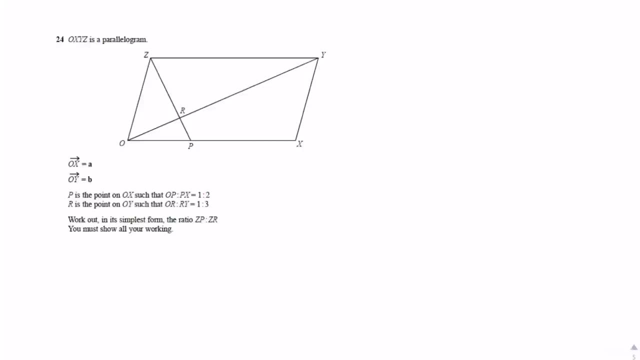 This one actually isn't too bad compared to the others. Just having a look at it now. So p is on the point 0x, such that o to p, p to x is 1 to 2.. So where is that? 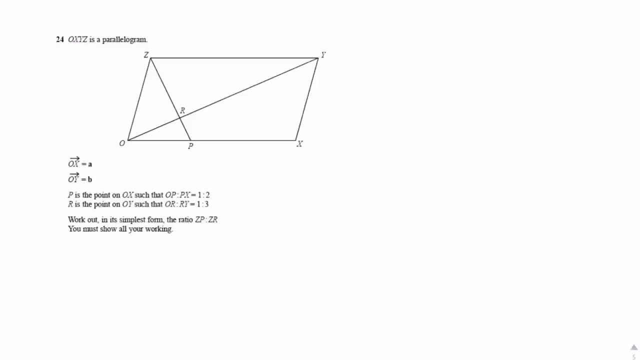 p to a. completely lost it there. o to p, p to x- there it is is 1 to 2.. So that's out of 3.. So that is 1.. 3rd, And this one here is going to be 2 thirds. 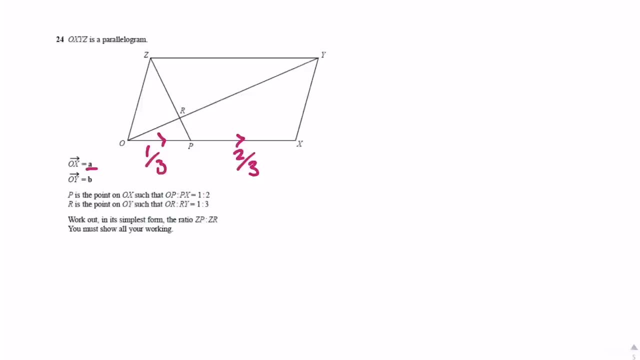 Now it says in the question that o to x is the vector a. It's given to us there. So that's the 3rd a and 2 thirds a. The next one it says o to y is the vector b. And then it tells us that o to y, such that o to r, r to y is 1 to 3.. 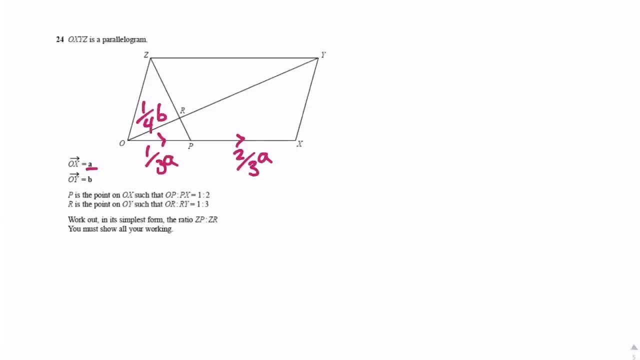 So that's out of 4.. So that's going to be 1 quarter, And again that's a quarter b moving in this direction. And there we go. the other one's going to be 3 quarters b. Now not forgetting obviously, this question says it's a parallelogram. 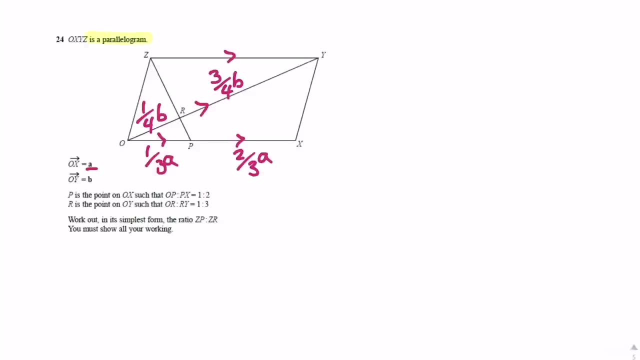 So the top vector here is going to be the same as the one at the bottom, So that's also going to be the vector a, And we may or may not need that. We'll have a look in a sec. So it says: 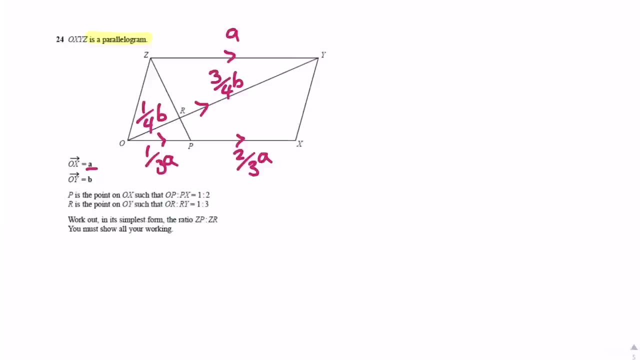 Where's z There? we go z to p, z to r, OK. so we're looking at this line here And that's our key line for the question: z to p, z to r, And you must show where you're working. 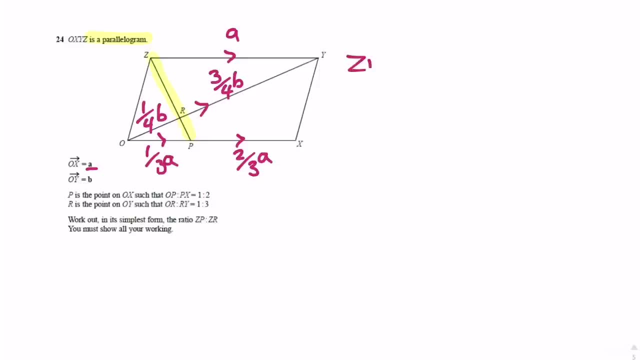 OK, so let's have a look Now. how do I get from z to p? Let's find the full length of that line: z to p. So z to p is Well. let's have a think how we could do that. 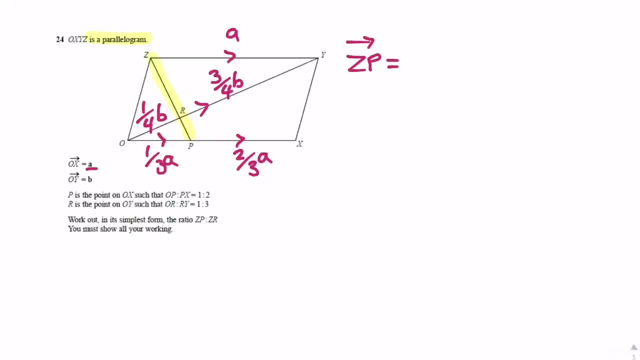 OK, So z to p, we can go from z to y, which is a, and then minus that 3 quarters b. So let's actually do that. then Let's go a minus 3 quarters b, Or is there another way that we could actually get there as well? 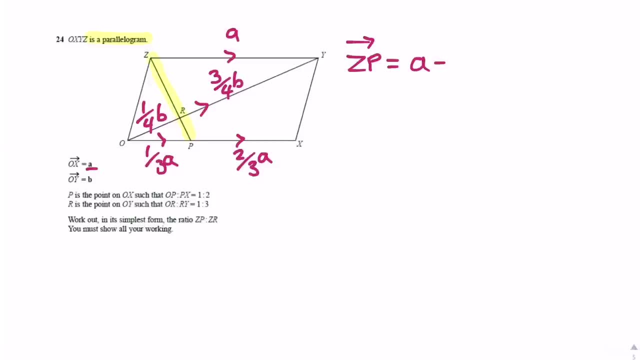 Oh yeah, we're doing the full length of the line, So we could actually get from z to r straight away. I just want to think about how we could approach this. Let's go for z to r straight away. We could actually get z to r and z to p. 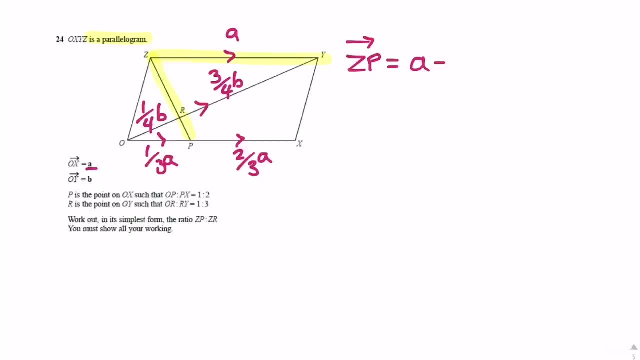 So z to r, we're going to go plus a And then minus 3 quarters b. Or, if we want to have a look at this, z to p, we could keep going. So all the way down the b and then a third of a. 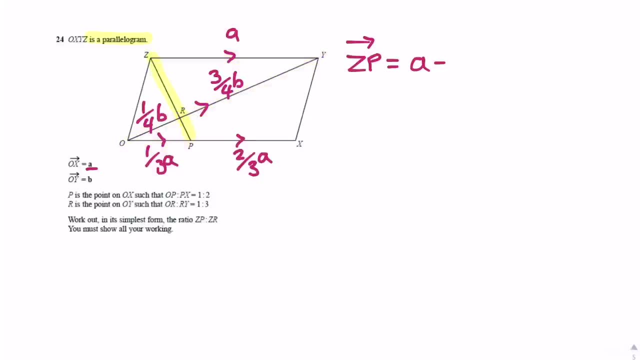 So let's do the full amount in the first go. Yes, that's the one I've written down. So from z to p, we've got a minus the full length of b. Add the third a. There we go. So in total that gives us one and a third a or four thirds a. 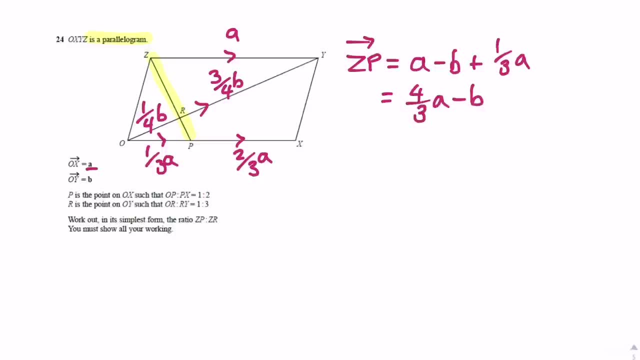 I'll just leave it as four thirds, Four thirds a minus b, And again we could factorise the third out Just to make it look a bit nicer. So if we factorise the third out, a third fits into four thirds four times. 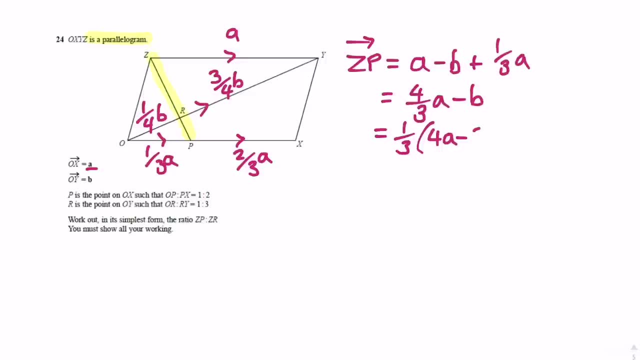 So four a, And it fits into b three times. So three b, So four a minus three b. There we go. There's a little vector for us Now, z to r, which I just almost did a second ago. We can get from z to r quite nice and easily. 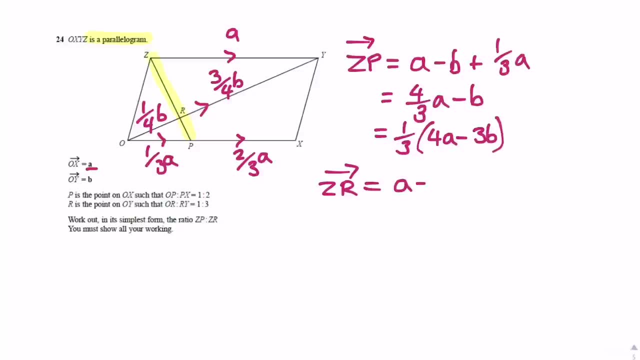 We go plus the a, from z over to y, And then minus the three quarters b. There we go, Minus three quarters b. There we are, And there is our vector there, And let's factorise that. Let's factorise a quarter out of this one. 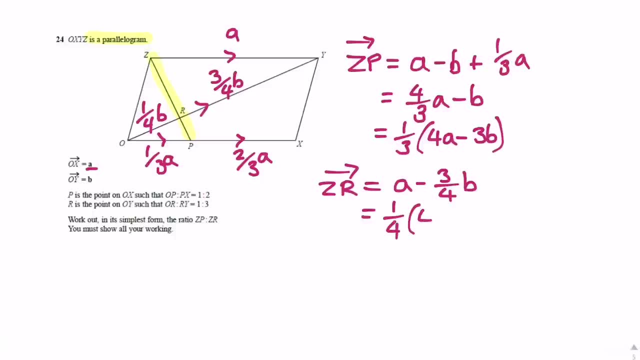 So a quarter, And that fits into a four times, And it fits into three quarters three times. So minus three b. Now at this point here, that's really nice Because we've got this matching vector there in the bracket. So for our final step, look. 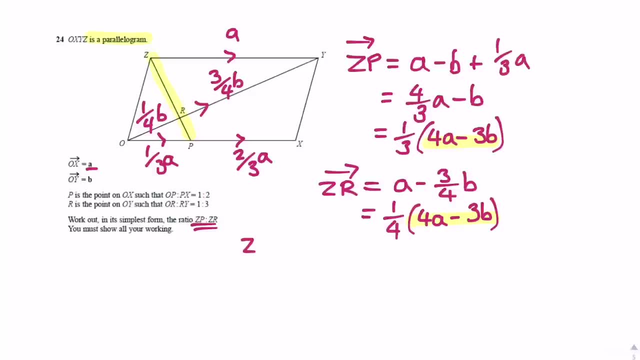 the vector z to p, z to r, which is what we're looking at. So z to p, which we've just found, Z to r, which we've also just found, At the moment is in the vector one third For z to p. 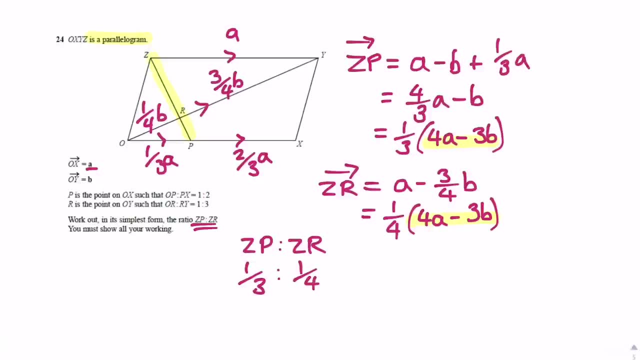 To one quarter. There we go, And obviously we just need to make these match. So, just like with normal fractions, let's make a common denominator. So we'll times this one by four, Make the denominator 12.. And we'll times this one by three. 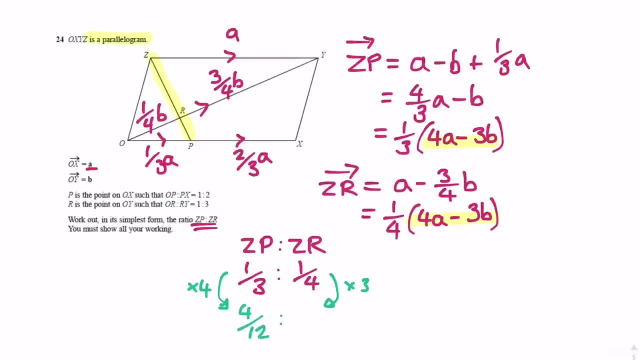 And that gives us four twelfths to three twelfths. Timesing both of those by 12 gives us the ratio four to three. So the ratio is four to three in its simplest form. There we go, And just gives that a bit of a highlight. 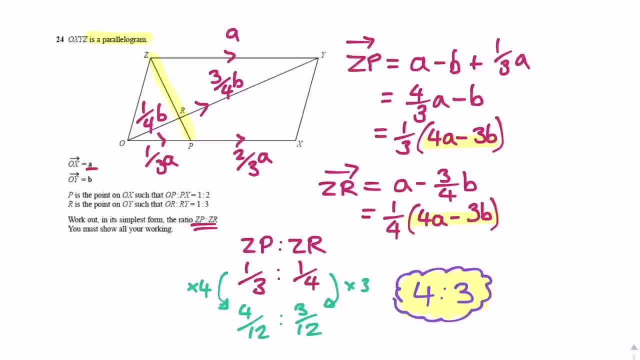 There we go, And there's our final question. Okay, obviously there's some pretty tricky questions there. That's quite a nice one to finish on. I've not done a huge amount of actually explaining the ins and outs of how and why for these particular questions. 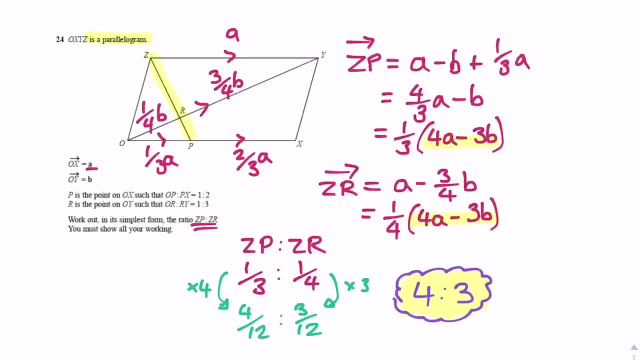 But I just wanted to make sure that obviously you had a little sort of way of actually getting a solution for these questions, because a lot of these are quite open and they are quite difficult. But there we go. That is sort of the five hardest vector questions that I've seen and, obviously, how to solve them. 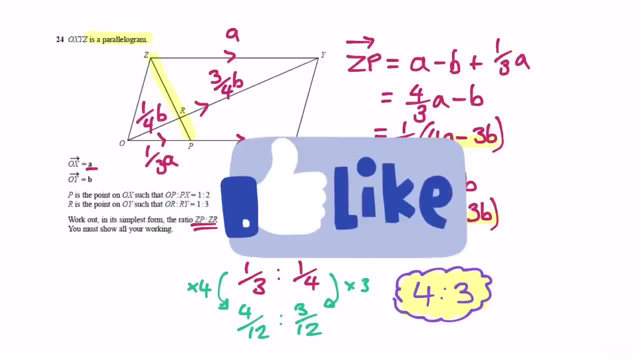 So hopefully that's helpful. Hopefully it's useful. If it was, please Obviously, please Like, please comment, please subscribe. Don't forget to check out the previous video on vector proofs. But there we go. That's the end of that one. I'll see you for the next one.